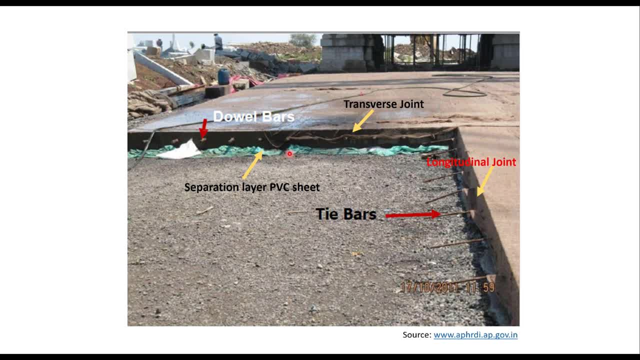 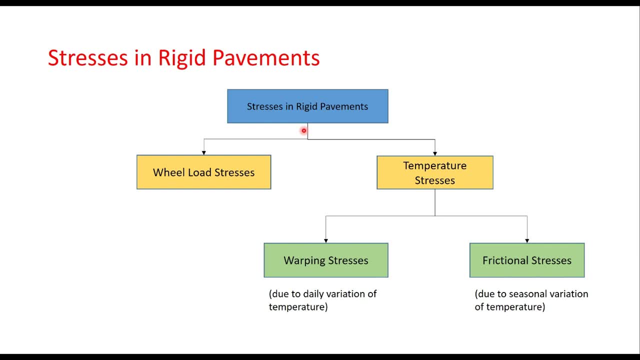 There is a separation layer which is a PVC sheet which is laid between the DL-C and the concrete slab. The stresses in rigid pavements are mainly because of V-load and temperature. The temperature can cause a lot of stress. It can cause burping stresses, which is due to daily variation in the temperature. 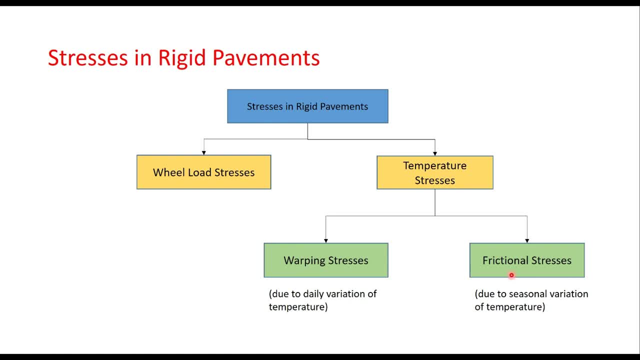 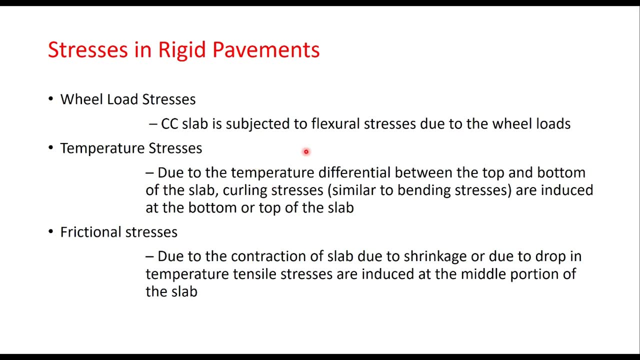 Or it may be frictional stresses which are due to seasonal variation of temperature. The V-load stresses create fragile stress in the slab And temperature stresses are due to the temperature differential between the top and bottom of the slab. That can create a curling stress which is similar to bending stress. 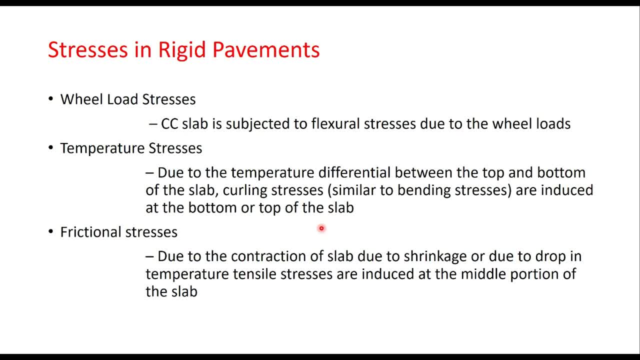 And this is introduced at the bottom or top of the slab, depending upon which part of the slab is hot. The frictional stresses occur because of contraction of the slab, which might occur due to shrinkage or due to drop in temperature, And that is also in the form of tensile stresses at the middle portion of the slab. 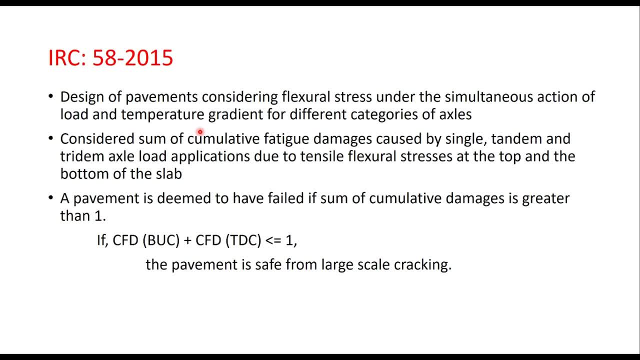 IRC 58 2015 considered design of pavement considering fragile stress under the simultaneous action of V-load and temperature gradient for different categories of the axles, And it takes into account the sum of cumulative fatigue damages caused by single tandem and tridem axle load applications. 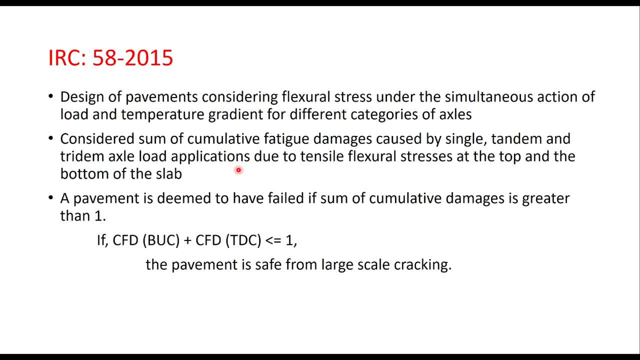 due to tensile flexural stresses at the top and at the bottom of the slab And a pavement is considered to have failed if some of the cumulative damages is greater than 1.. If the cumulative fatigue damage because of bottom up cracking plus cumulative fatigue damage because of top down cracking is less than or equal to 1,. 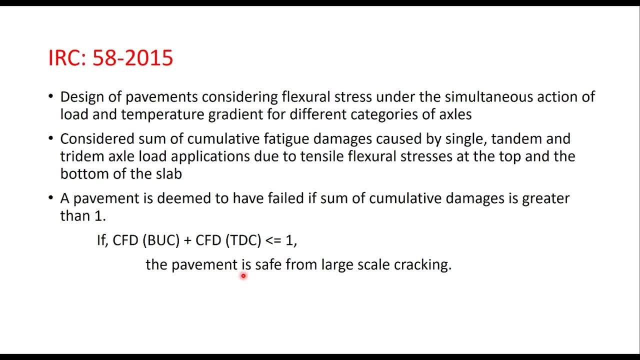 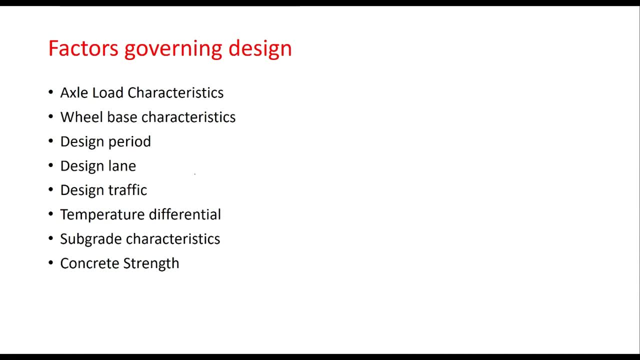 then the pavement is considered to be safe from large-scale cracking. There are several factors which govern the design of a concrete pavement. These include axle load characteristics, wheel load, wheel base characteristics, design period design, lane design, draft temperature, differential subgrade characteristics and concrete strength. 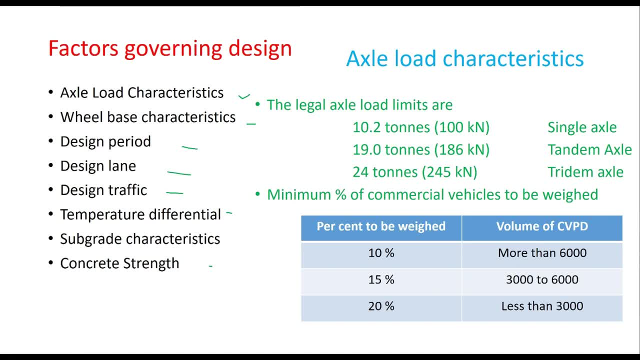 When it comes to axle load characteristics, the legal axle load limits in India are 10.2 tons for single axle, 19 tons for tandem axle and 24 tons for tridem axle. It is important to carry out axle load survey in field to get the overloading spectrum on the pavement. 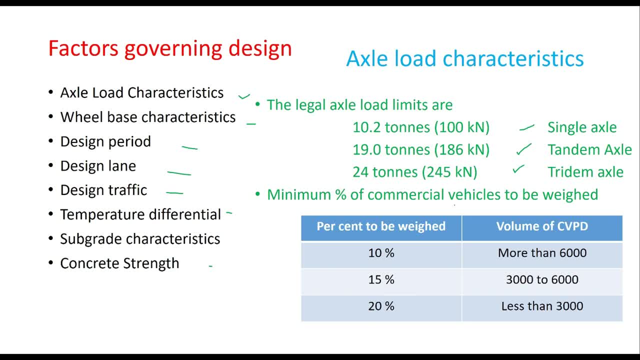 because the design of the pavement is based on cumulative fatigue analysis And therefore concept of pavement is based on cumulative fatigue analysis And therefore concept of pavement is based on cumulative fatigue analysis. VDF is not applied here, and when we carry out excel load survey, the sample size that should. 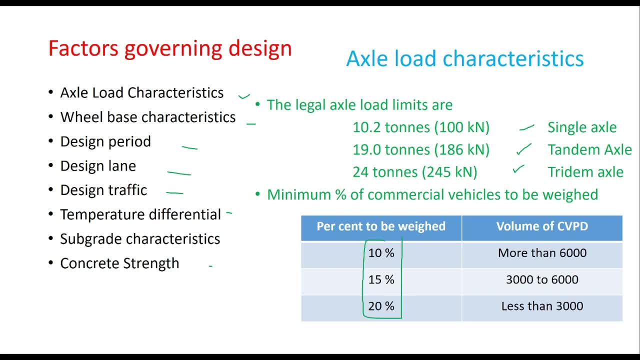 be taken. that depends upon the number of commercial vehicles per day. For more than 6000, at least 10% should be weighed. for 3000 to 6000: 15%. and for less than 3000 CVE per day, at least 20% of the. 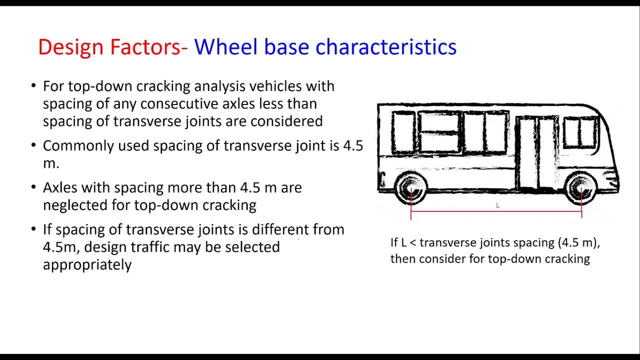 sample size should be taken. As regards to wheelbase characteristics, a rigid pavement is analyzed for top-down cracking and as well as for bottom-up cracking. For top-down cracking, excels having spacing less than or equal to 4.5 meter are only considered, and this 4.5 meter. 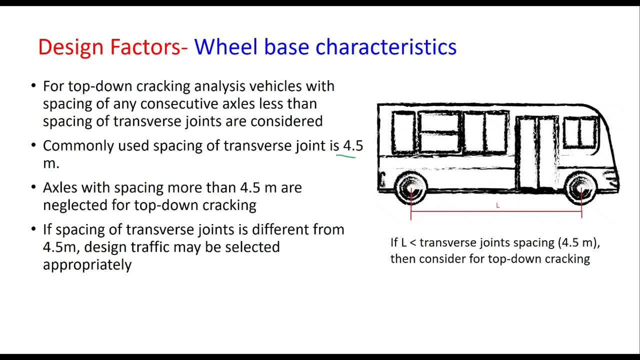 is considered because this is the typical spacing between transverse joints. Excel with more than 4.5 meter are not considered in case of top-down cracking and if the spacing of transverse joint is different from 4.5 meter, then design traffic is not considered. 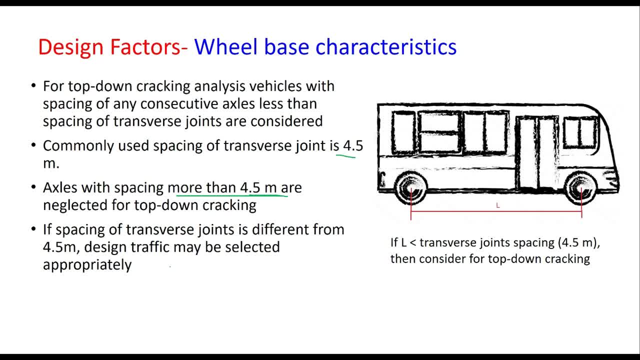 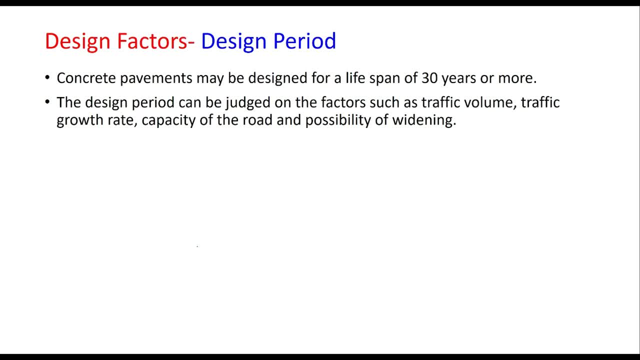 The design life. the concrete pavements are designed generally for 30 years, but the design period may change depending upon the factors like traffic volume, traffic growth rate and capacity of the road and possibility of widening at later stage. Design lane: the lane carrying maximum. 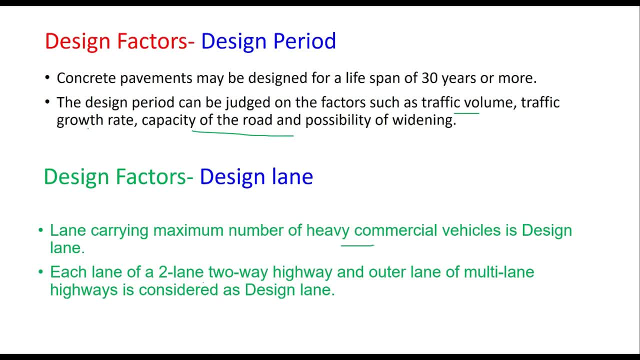 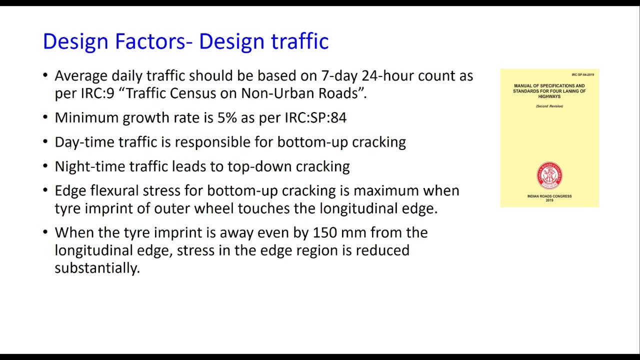 number of heavy commercial vehicles is considered the design lane, and this will be each lane of a multi-lane two-way highway and the outer lane of multi-lane highway is considered as design lane. Now design traffic should be calculated based on average daily traffic counted for seven days, 24. 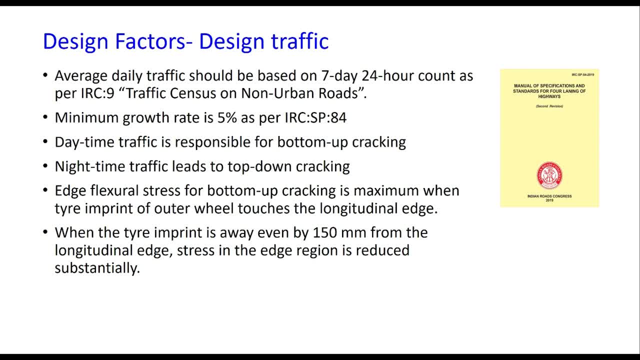 hours as per guidelines, given the IRC 9.. As far as possible, growth rate should be estimated from past data, but IRC SP 84 suggests a minimum growth rate of five percent. Day time is responsible for bottom-up cracking and night-time traffic leads to top-down cracking. 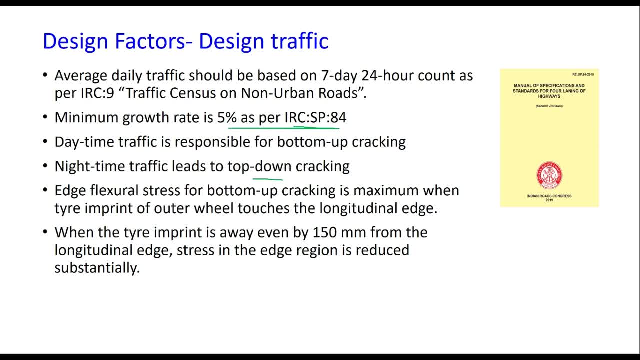 Edge flangele. stress for bottom of cracking is maximum when tire imprint of outer wheel touches the longitudinal edge. When the tyre print is away, even by 150 millimeter from the longitudinal edge, the stress in the edge region is reduced substantially. Typical lateral distribution. 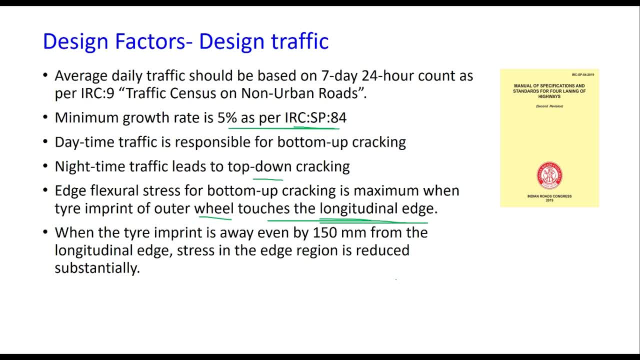 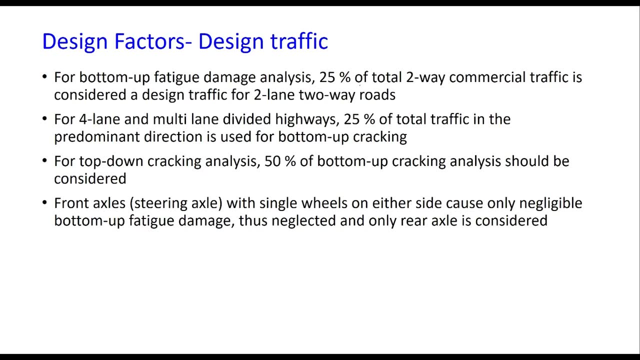 characteristics of wheel path of commercial vehicles observed on Indian highways indicate that very few wheels of vehicle are tangential to the longitudinal joints And therefore for bottom of fatigue damage. 25% of total two-way commercial traffic is considered as design traffic for two-lane, two-way roads. 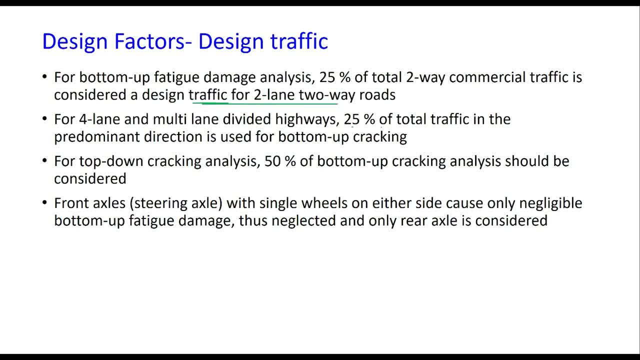 For four-lane and multi-lane divided highway, 25% of total traffic in the predominant direction is used for bottom-up cracking. For top-down cracking analysis, 50% of bottom-up cracking analysis is taken And the front axles with the single wheel on either side will cause very little bottom. 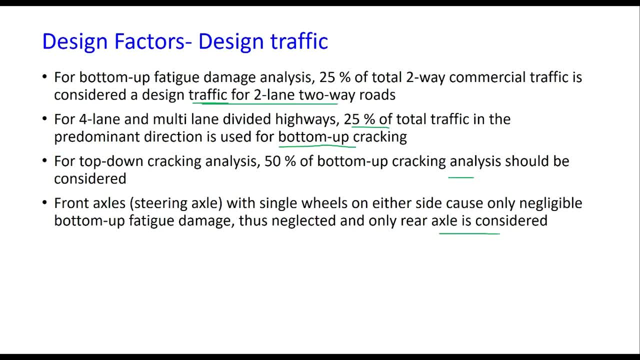 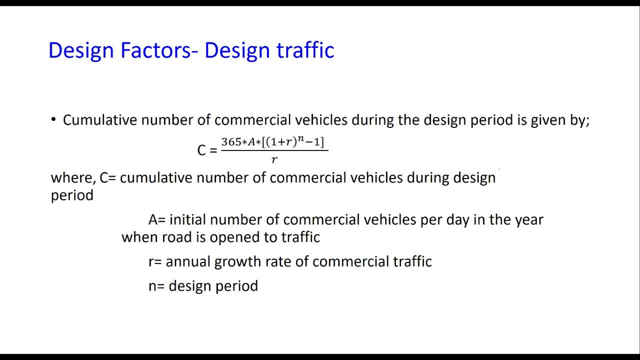 of fatigue damage and therefore they are generally not considered in the design. Design traffic is calculated as by normal equation, given here: 365 × A 1 plus R, power, n minus 1 upon R. R is the growth rate. A is the initial number. 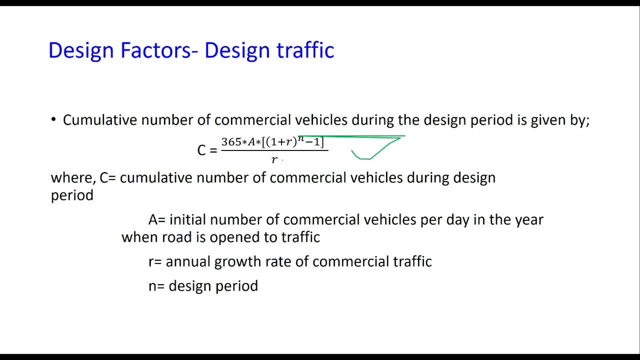 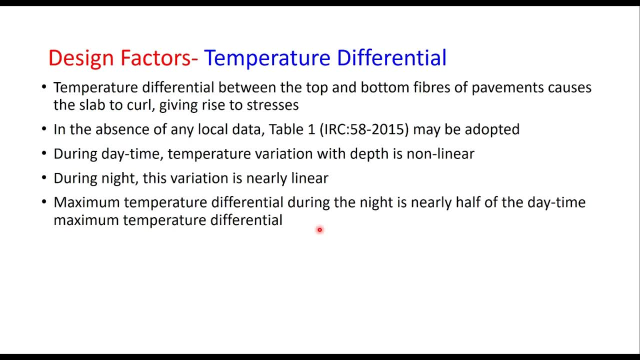 of commercial vehicles per day in the year when the road is open to traffic. Another important design factor is temperature differential between the top and bottom fibers of the pavement, And that can cause the slab to curve, giving rise to stresses. The temperature gradient in a concrete slab depends upon several factors like longitudes. 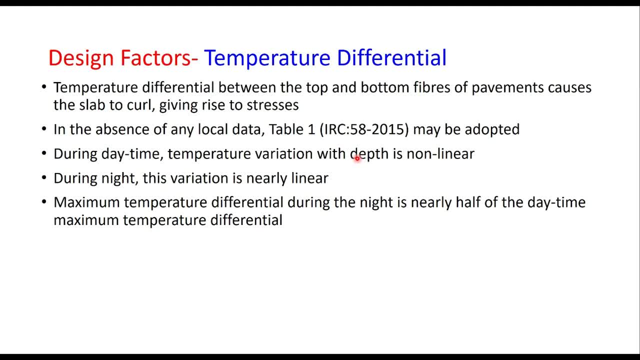 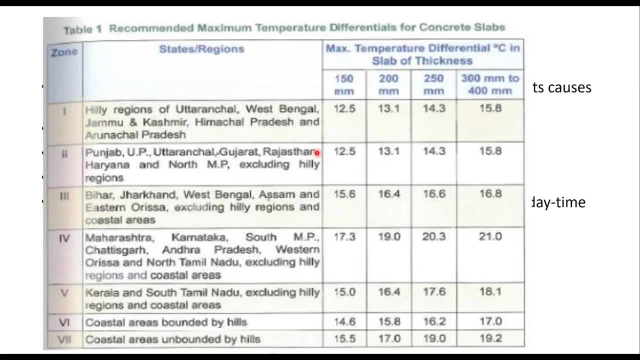 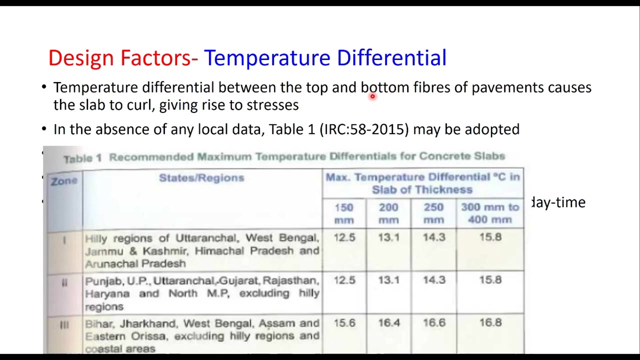 and latitude of the area, and it must be estimated for the given situation. In the absence of local data, a table given in IRC 58 can be used to take the maximum temperature differential. In the absence of local data, a table will be used to calculate Points of Calculation. 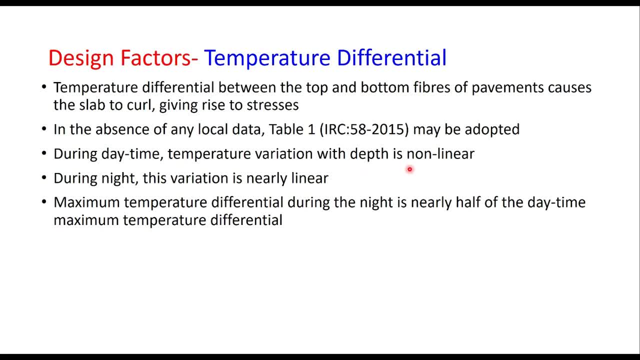 of details, for example the given Assessment of temperature, stress and number of dipoles. My first slide is showing the temperature variation between areas used for the pavement and the deeper slab And for conveying. thoseSí make the line uniform. 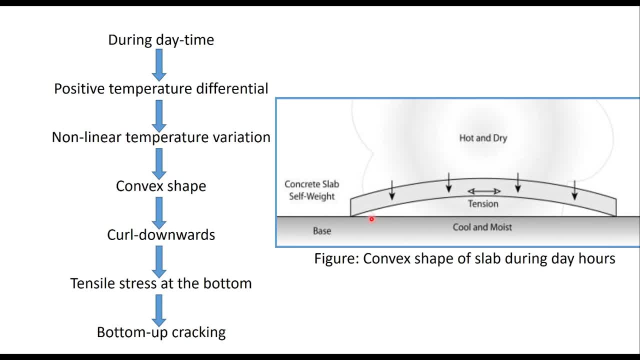 The beginning embossed slab starts to curve. The slope makes the bank ten degrees above and supports the base. when the top surface of the pavement slab is hotter than the bottom surface- and it happens during daytime- and this gradient is nonlinear, creating bending or curling in the slab downward. that creates tensile stresses at the bottom. 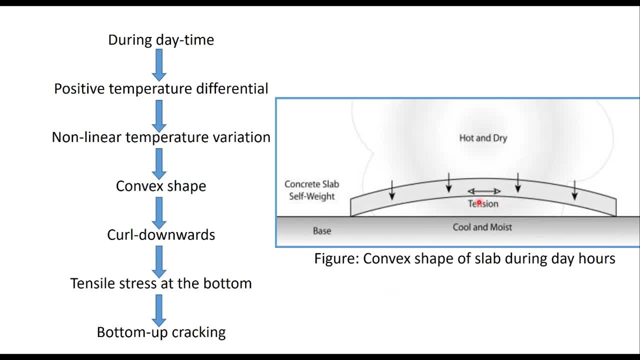 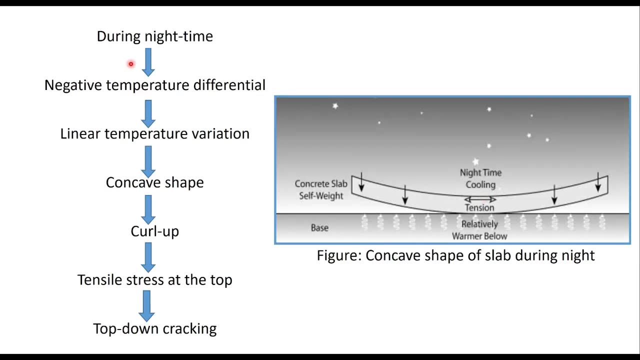 and this becomes in tension. this side of the slab becomes in tension and crack may initiate at the bottom and then they can propagate upward, and that is called bottom of cracking. during nighttime there is a negative temperature differential which is taken as linear and therefore the slab will take. 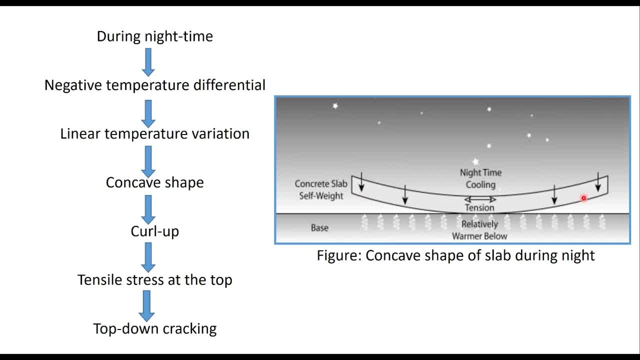 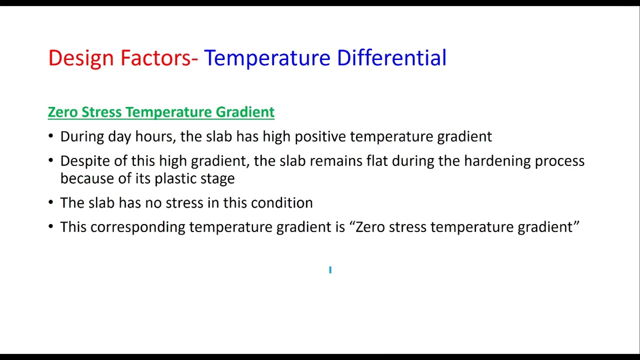 the concave shape curling upward and tensile stress will develop at the top. and when the wheel comes on this pavement the tensile stress will behave and there will be a crack on the top of the slab and it will propagate downward. another important consideration: in temperature. 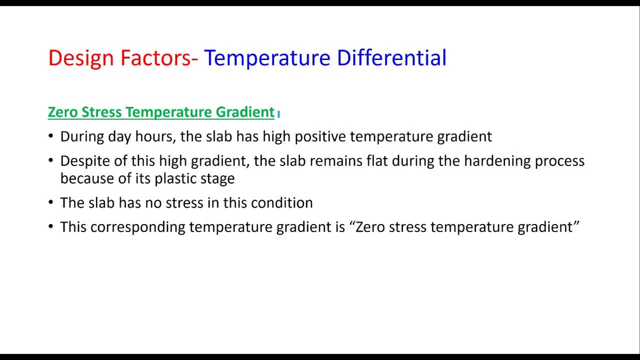 gradient is zero stress temperature gradient. concrete pavements in India are generally laid during night hours due to high temperature during daytime, and therefore a slab laid during night will experience high positive temperature gradient and will experience a good amount of tension during daytime, during daytime. But despite of this high gradient, the slab remains flat during the hardening process. 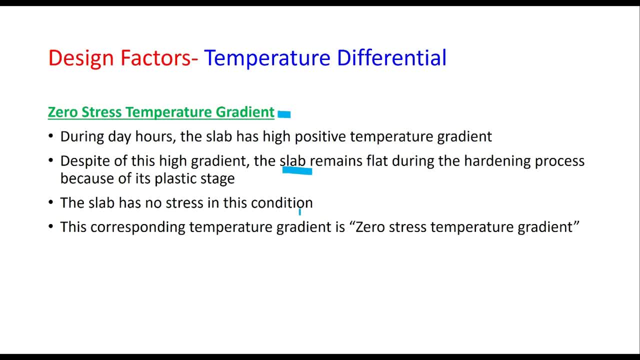 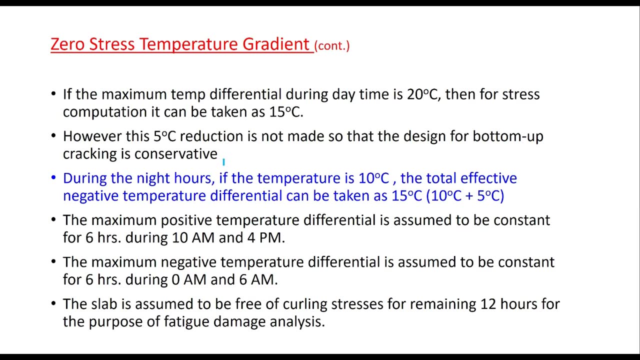 because of its plastic stage And during this condition, slab has no stress. And this temperature gradient- when there is no stress in the slab- is called zero stress temperature gradient. Now, research indicates that exposure of fresh concrete to sun during hardening process 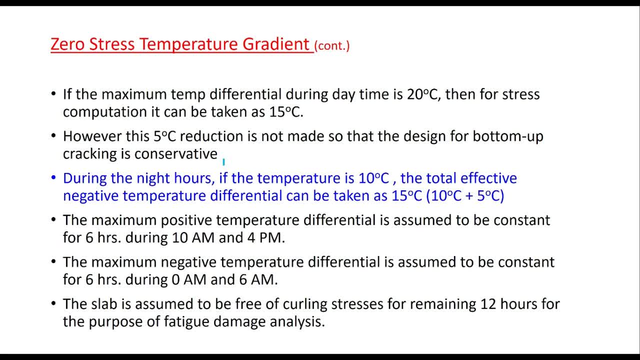 causes a permanent curve in the concrete pavement, And this curve is nearly equal to the curve caused by a negative temperature differential of 5 degrees centigrade. And therefore, when the maximum temperature differential during daytime is 20 degrees centigrade, then for the purpose of stress calculation it can be taken as 15 degrees centigrade. 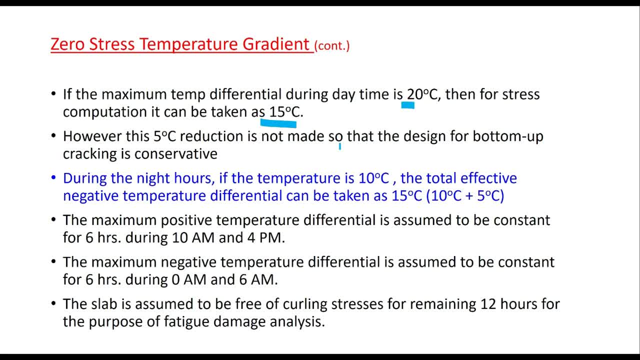 However, this reduction is not made so that the design for bottom-up cracking is consistent. But during night hours, if the temperature is 10 degrees centigrade, then total effective negative temperature differential can be taken as 15 degrees centigrade The maximum positive. 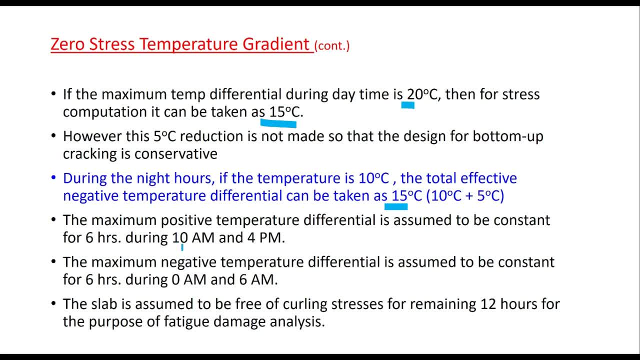 temperature differential is assumed to be constant for six hours during 10 am and 4 pm, And the maximum negative temperature differential is assumed to be constant for six hours from midnight to 6 am in the morning, And the slab is assumed to be free of curling stresses for the remaining 12 hours for the purpose of fatigue damage analysis. 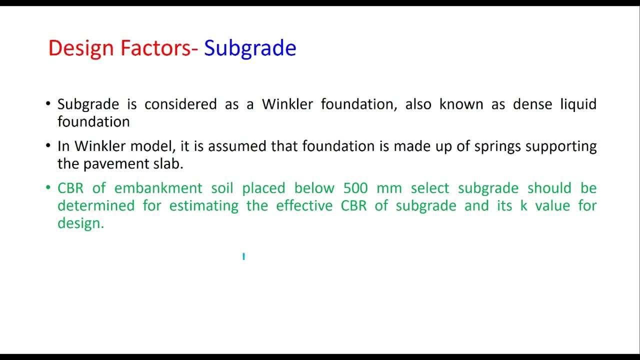 Another important consideration in the design is the strength of the subgrade, And in concrete pavement analysis, subgrade is considered as a regular foundation, which is also known as dense liquid foundation. Here it is assumed that foundation is made up of springs supporting the pavement slab. 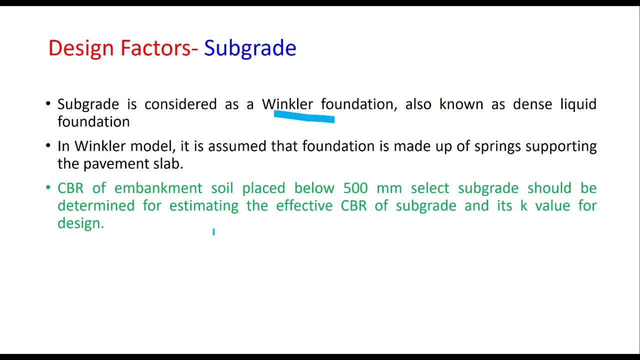 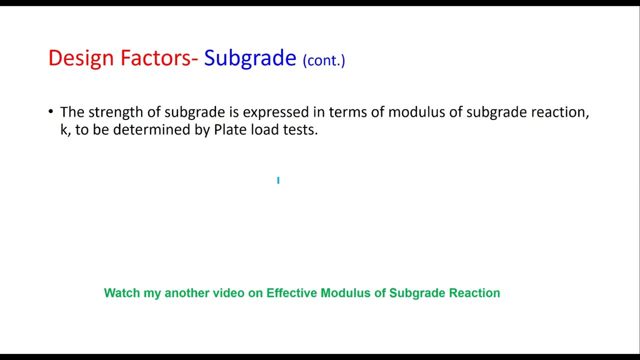 The CBR of the cement soil placed below 500mm subgrade should be determined. for estimating the effective CBR of subgrade and its K value for design, The strength of subgrade is expressed in terms of modulus of subgrade reaction, which is K, And it is determined by plate load test. 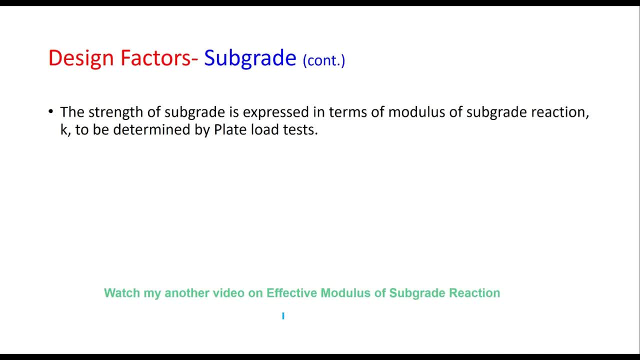 And you can watch my another video on effective modulus of subgrade reaction. The IRC 58 suggests the relationship between Brasiló and Israel is 36 Владigr stud. the Rc 58 suggests the relationship between captureson experience and T trial of subgrade-reaction changes. 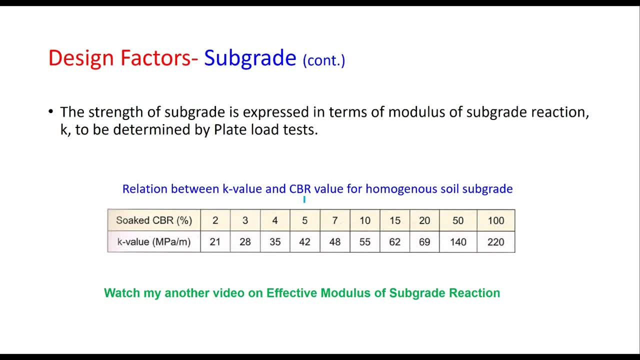 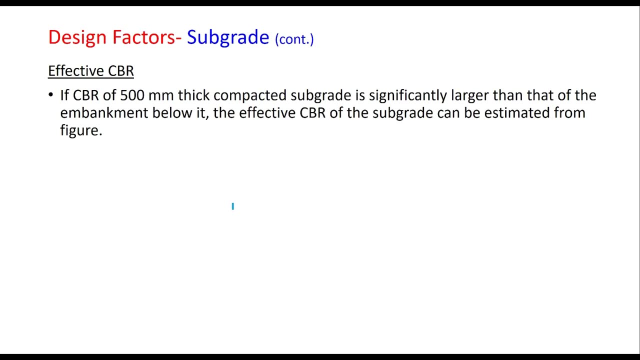 and proceed. a wanna be responsible. K value and CBR for homogeneous soil subgrade and you can choose the value of K for a given effective CBR of subgrade soil If the CBR of 500 millimeter thick compacted subgrade is significantly larger than that of a magnet below the 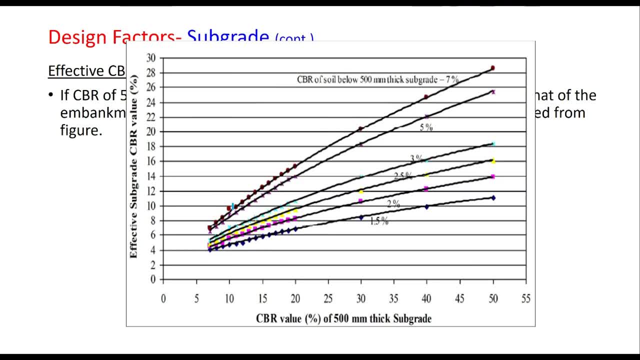 effective CBR of subgrade can be estimated from this figure, And this figure gives you the CBR value of 500 millimeter thick subgrade and the CBR of soil below 500 millimeter thick subgrade, that is, that is, the CBR of a. 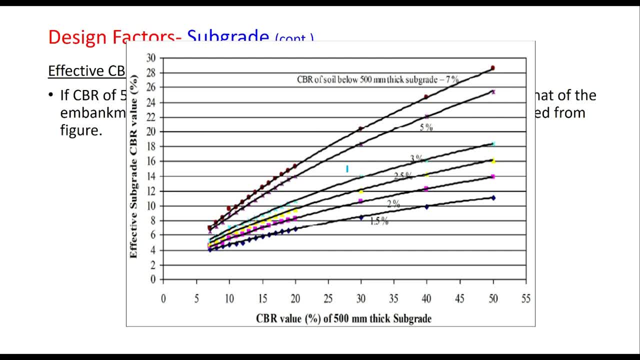 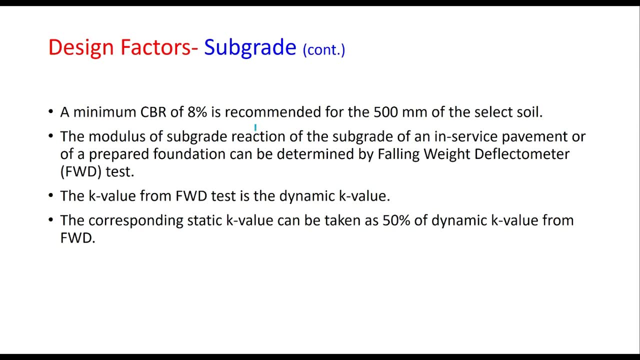 magnet soil And corresponding to these two values, you can find out what is the effective subgrade CBR. Now this procedure is similar to what I explained in the design of flexible pavement using IRC-37.. A minimum CBR of 8 percent is recommended for the 500 millimeter thickness of subgrade soil and the modulus of 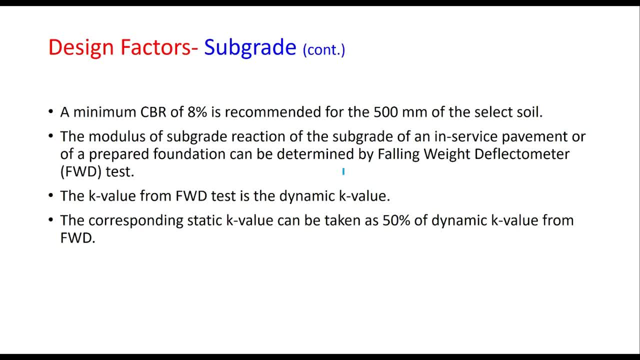 subgrade reaction of the subgrade for an in-service pavement or of a prepared foundation can be estimated by falling weight deflectometer. but we should remember that the value of k, which is determined from fwd data, is dynamic k value and for design purpose the static k value should be. 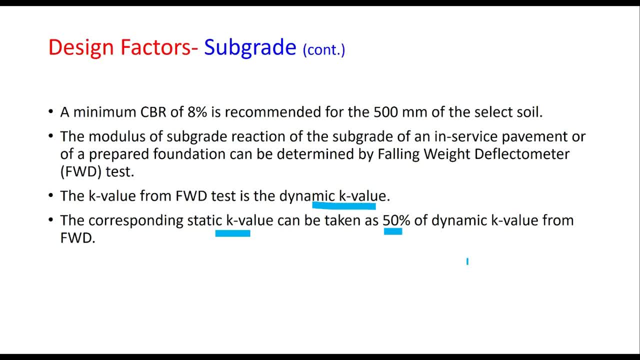 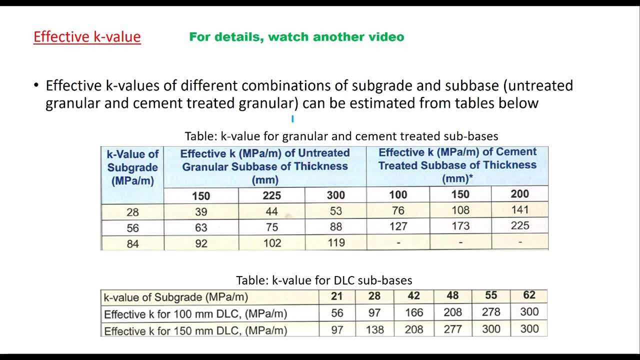 taken as 50 percent of dynamic k value. in the absence of fwd data, k value can be determined for different combinations of subgrade and sub base, for treated and untreated, from this table. alternatively, you can watch my video for estimating the effective k value of subgrade reaction. 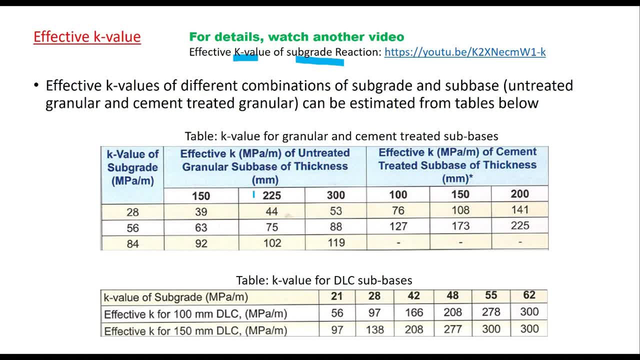 now this table gives you k value of granular and cement treated sub base for different thicknesses of sub base layer, and this is the k value of subgrade soil. you can choose the value of effective k from this table if dry lean concrete is provided as sub base material. 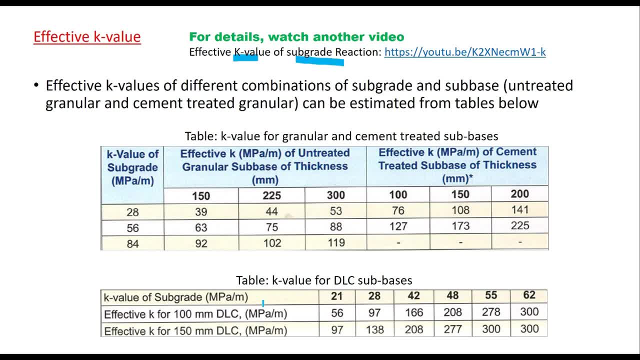 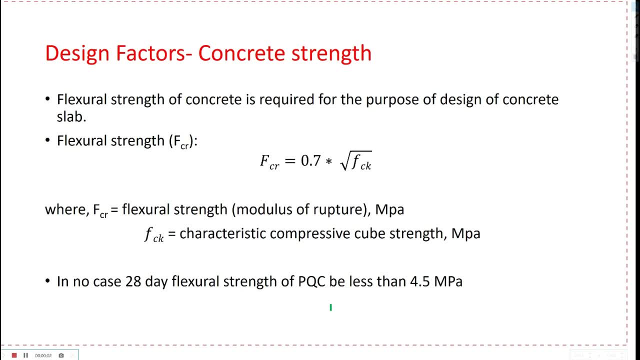 then, depending upon thickness of the dlc layer, you can find out the k value of subgrade. the last factor in the list of design is the concrete strength, and the pressure strength of concrete is required for the purpose of design of concrete pavement. the pressure strength can be estimated from the characteristic strength of the concrete. 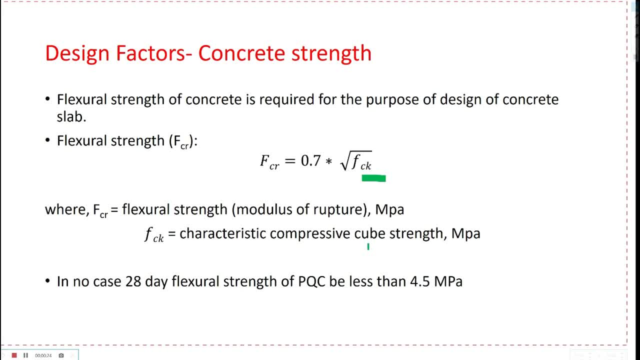 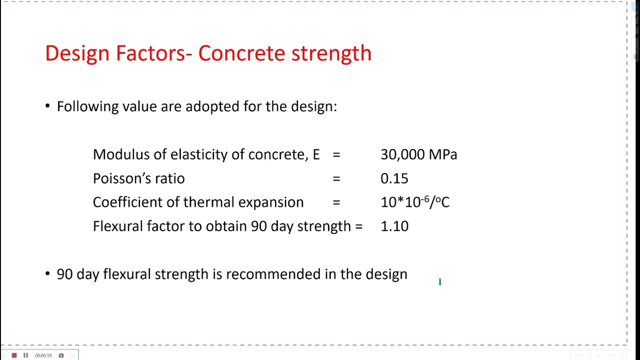 which is the 28 days cube strength and what irc code suggests that in no case this 28 days pleasure strength of pavement quality concrete be less than 4.5 mpa? the default values of concrete which are given in the code are models of elasticity of concrete. 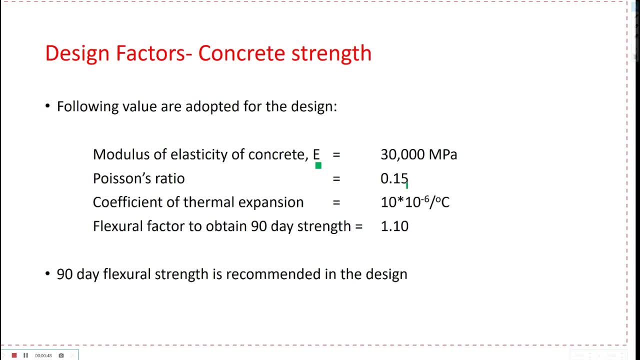 e value, that is 30 000 mpa. ocean ratio can be taken point 1: 5, coefficient of thermal expansion: 10 to the power minus 5 per degree centigrade and pressure factor to obtain 90 day strength is 1.10. 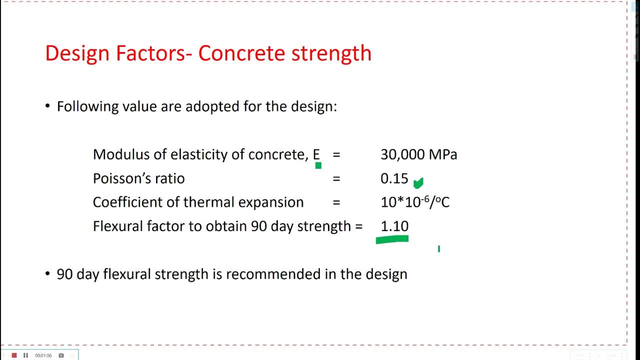 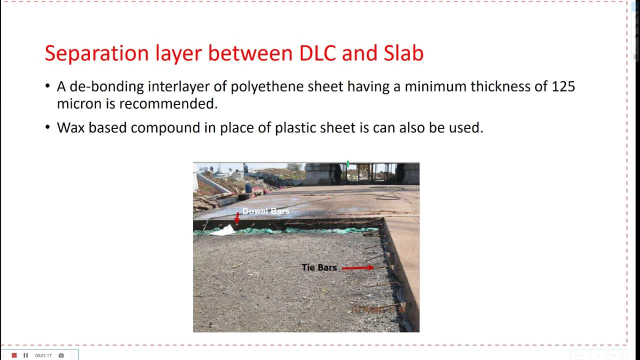 90 days pressure strength is recommended. in the design, the interface layer between the concrete slab and the dry lean concrete layer can be made smooth to reduce the inter layer friction and for this purpose a debonding layer of polythene sheet having a minimum thickness of 125 micron is recommended. alternatively, wax based compound. 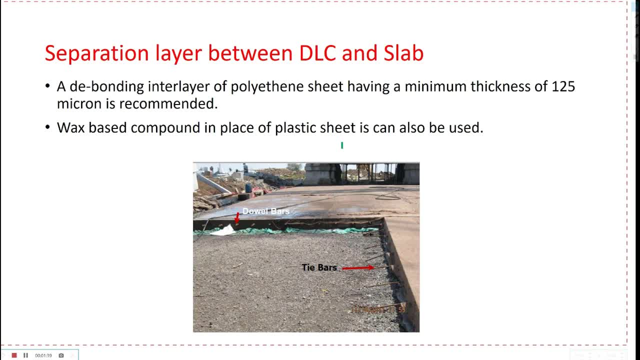 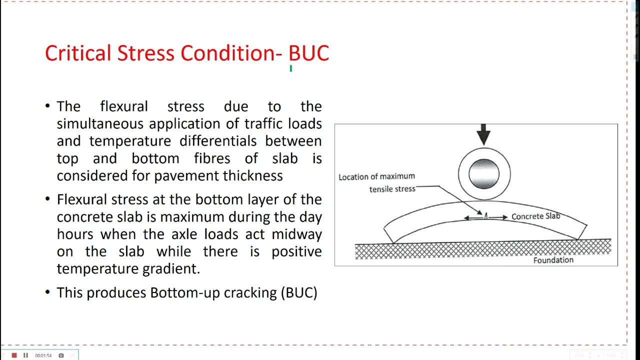 can also be used, or a layer of bitumen scrubbing material. concrete with grading 2 can be another option for this purpose. There are two critical conditions which are to be considered in the design of concrete slab. One is bottom up cracking and another one is top down cracking. 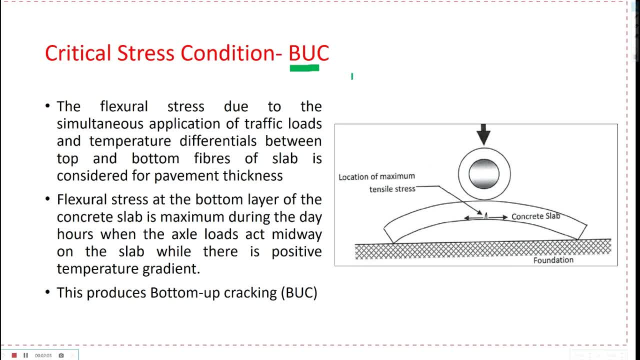 Now bottom up. cracking occurs during day time, when the temperature gradient is positive and the slab takes the shape of the curve like this, and the wheel load is at the center of the slab. Now this gives the critical condition of lateral stress and the stress at the bottom fiber of the concrete slab. 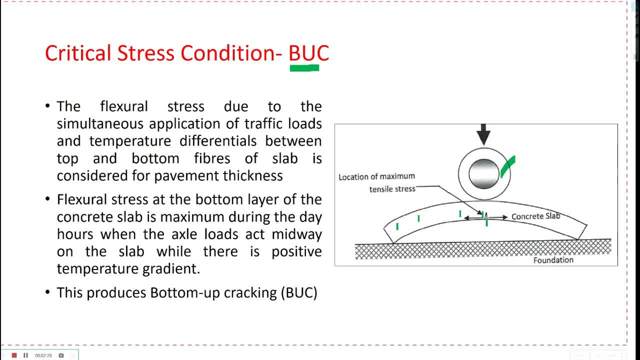 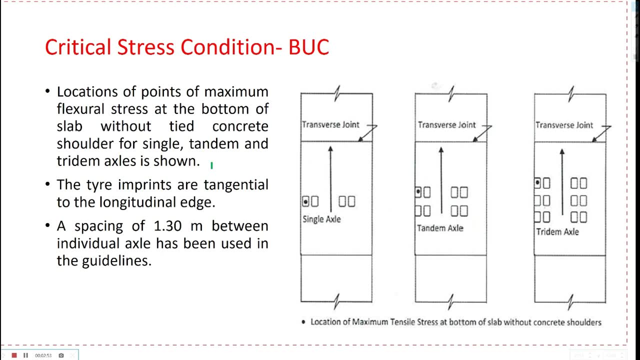 is maximum and that can trigger a crack at the bottom and it will propagate upward and this procedure is called bottom up cracking. Location of points of maximum pressure stress at the bottom of slab without tied concrete shoulder for single tandem and tridem axle is shown in these figures. 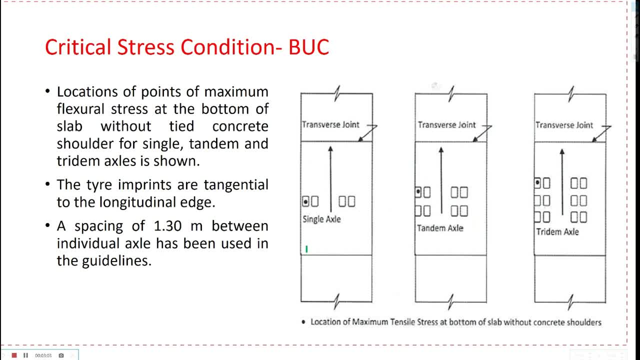 The tire imprints are tangential to the pavement edge and the spacing between individual axles for tandem and tridem axles vary from 1.3 meter to 1.4 meter and practically there is no difference in stresses for axle spacing of 1.3 meter or 1.4 meter and therefore a spacing of 1.3 meter. 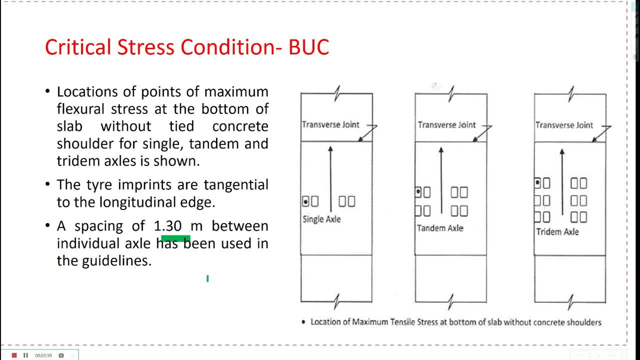 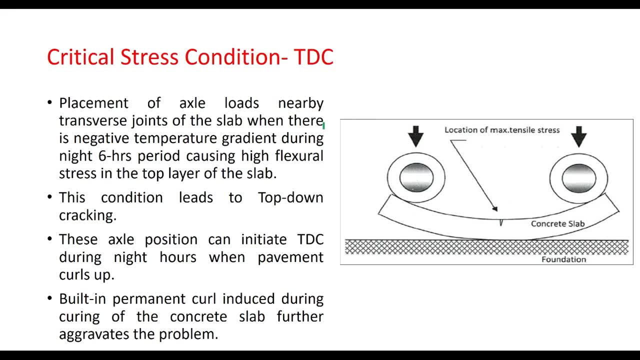 between individual axle has been used in the guidelines. During night hours, the top surface is cooler than the bottom surface and the slab will curve upward in a concave shape. The self weight of the slab and the resistance provided by the double bar will create tensile stress at the top of the slab. 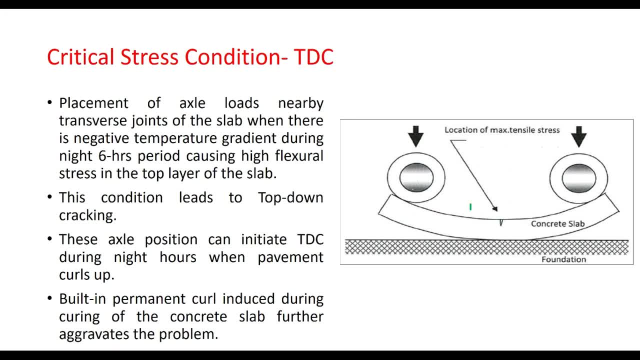 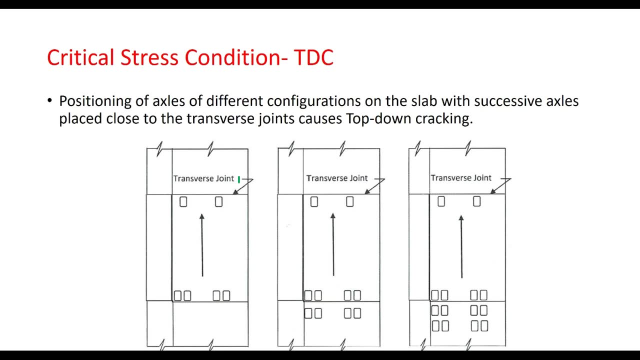 The axle load which is placed to the close to the transverse joints during night period will further increase the flagellary strength in the top layer, leading to a situation of top down cracking A position of axles of different configurations on the slab with successive axles. 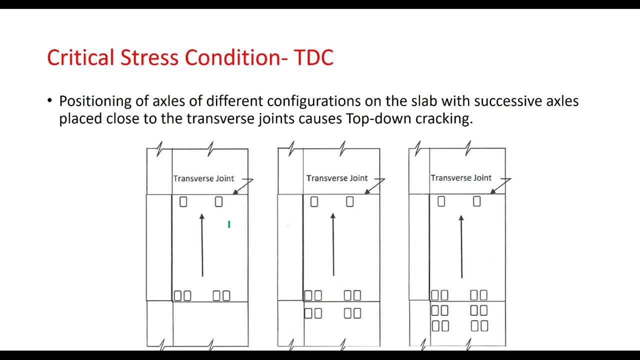 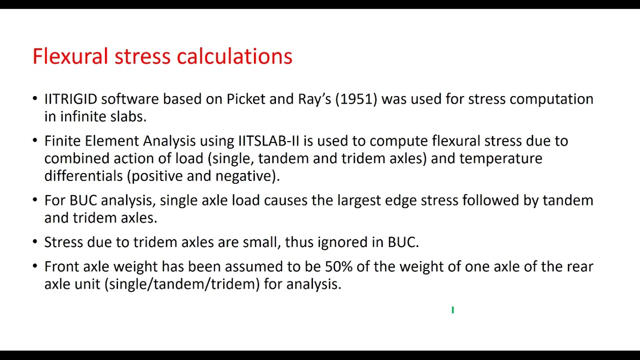 should be like this: for top down cracking to occur, The axles should be very close to transverse joint in case of single axle, double axle or tridem axles. The IIT rigid software based on picket and ray is used for stress computation in infinite slabs. 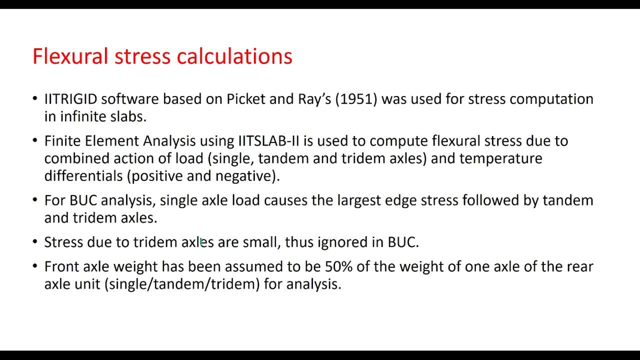 and for bottom up cracking, the single axle load causes the largest edge stresses, followed by tandem and tridem axles. The stresses due to tridem axles are very small and therefore they are ignored in bottom up cracking analysis, and front axle weight has been assumed to be 50 percent of the weight of one axle of. 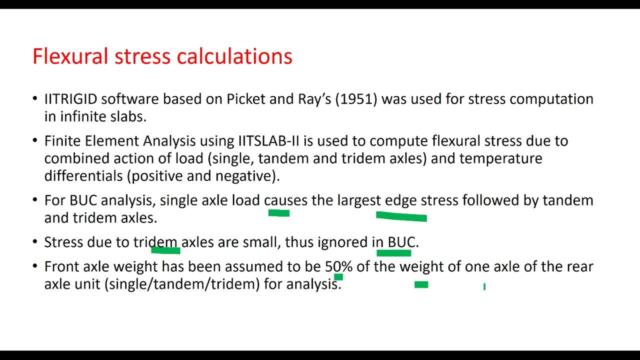 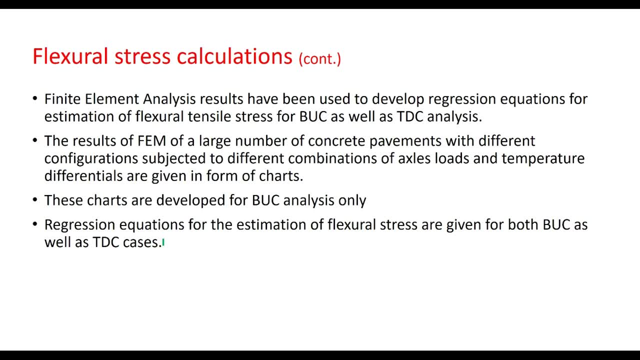 the rear axle unit for single, tandem or tridem for the purpose of analysis. The finite element analysis results have been used to develop regression equations for estimation of residual transile stress for BUC as well as for TDC analysis, and several charts are developed for. 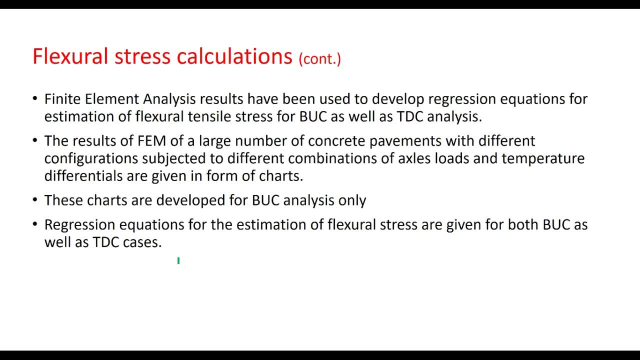 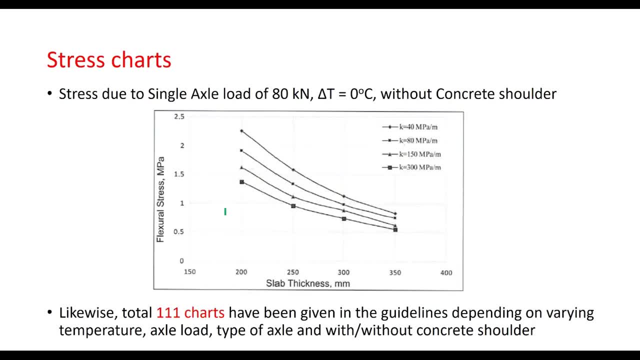 BUC analysis and for TDC for top down cracking analysis, the regression equations are suggested in IRC code. This is just one chart with the axle load of single axle load of 80 kilo Newton. The regression equation of top down cracking is developed as follows: 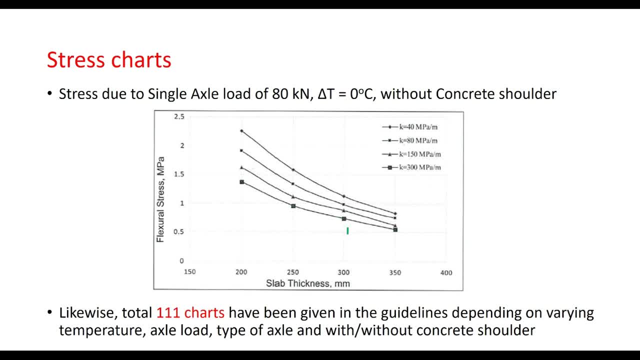 The regression equations for the top down cracking are set to base on the slope of the edge of the axle or the vertical slope of the axle, and the tension of the axle will be the trajectory and the angle of the axle. These are called TDC equations and these are defined by the. 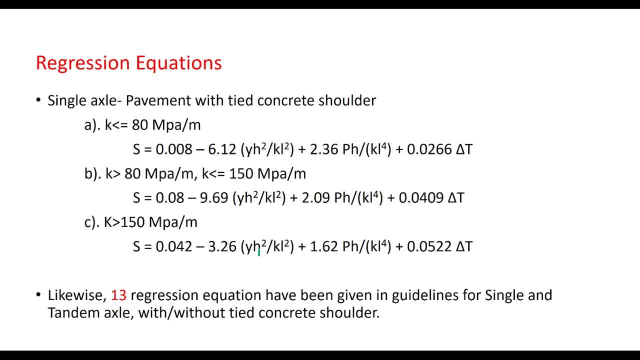 movement of the axle load with a constant force. For this reason, it is often used for testing the past cycle, the total temperature and the temperature gradient of zero degree centigrade, without any concrete shoulder, and for different values of K. Likewise, there are 111 charts in IRC code depending upon varying temperature, axle load, type of axle and with or without concrete shoulders. Similarly, the regression equations for top down cracking are developed like this: 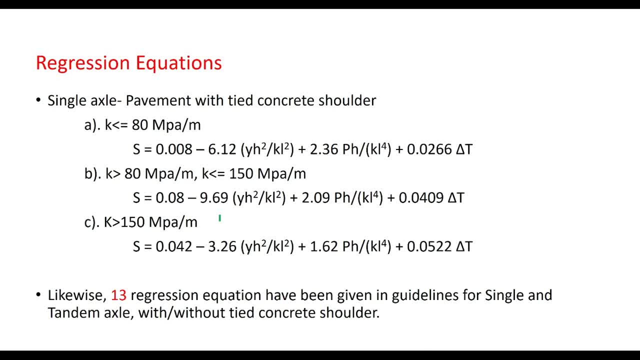 These are the current calculations for top down cracking of the axle load and the tension in the axle load if you consider the two angles in the axle load. just one example. and likewise there are 13 such equations given in the guidelines for single tandem axial, with or without tied concrete shoulder. 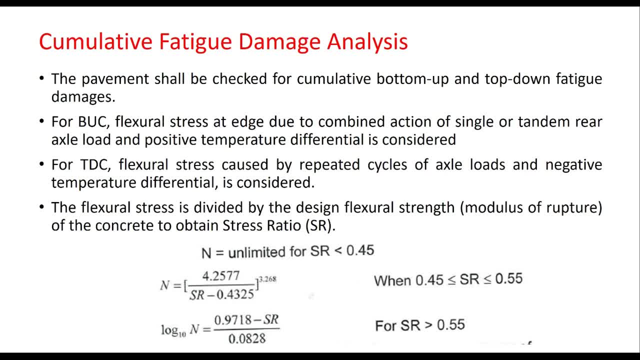 The design is based on cumulative fatigue damage analysis of concrete slab due to wheel loads of different magnitudes and also temperature gradient. The pavement is checked for cumulative bottom-up and top-down fatigue damages. For bottom-up, cracking, flexural stress at the edge due to combined action of single or tandem rear axial load and positive 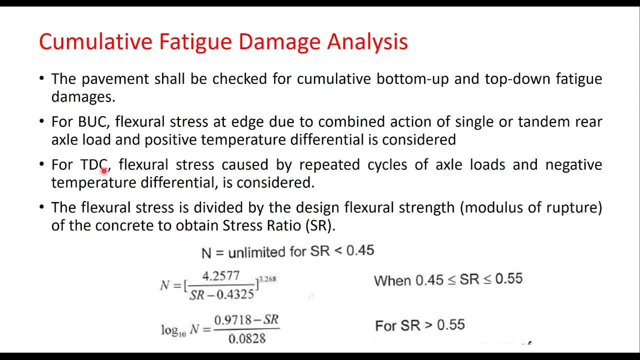 temperature gradient is considered and for top-down cracking it is negative temperature differential. plus stress is caused by axial loads. This flexural stress is divided by the design flexural strength that is, modulus of rupture of concrete to operate on the surface of the concrete slab. This flexural stress is divided by the design flexural strength that is modulus of rupture of concrete to operate on the surface of the concrete slab. 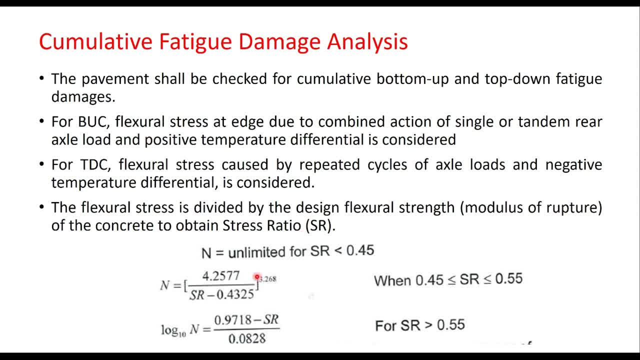 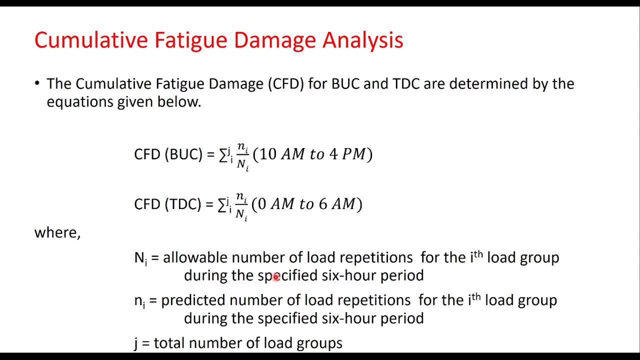 structure bounced off by axial loads. as I told you earlier, buc is considered when temperature gradient positive and it occurs during 10 am to 4 pm in daytime and therefore cumulative fatigue damage for bottom up cracking is considered for traffic from 10 am to 4 pm and this is the cumulative damage. 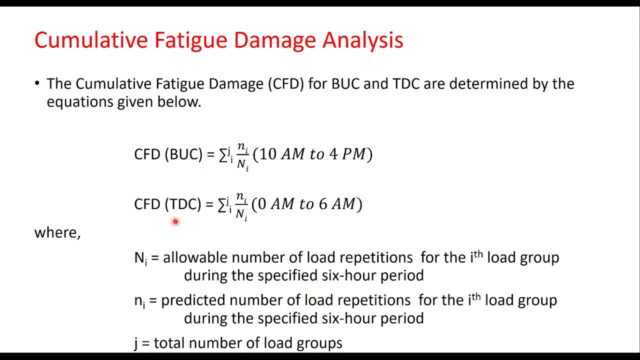 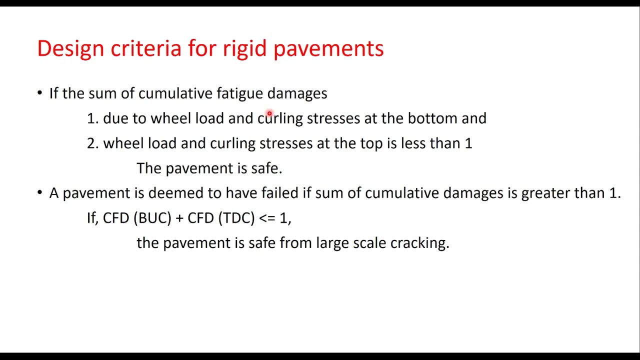 Similarly, cumulative fatigue damage for top-down cracking is considered for the time period from midnight to 6 am in the morning. The design criteria for rigid pavement is that the sum of cumulative fatigue damages should be less than or equal to 1.. 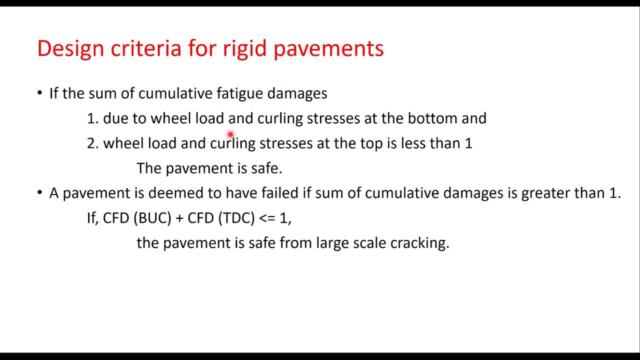 Now this fatigue damage due to wheel load and curling stresses at the bottom and the fatigue damage due to wheel load and curling stresses at the top. The sum should be less than 1.. Then the pavement is safe. In other words, if CFD of bottom-up cracking case plus CFD for top-down cracking case is less than or equal to 1,. 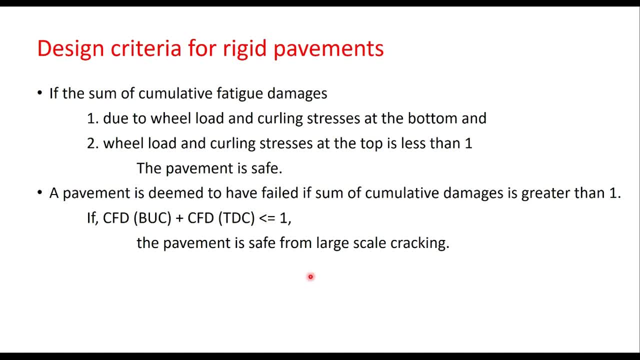 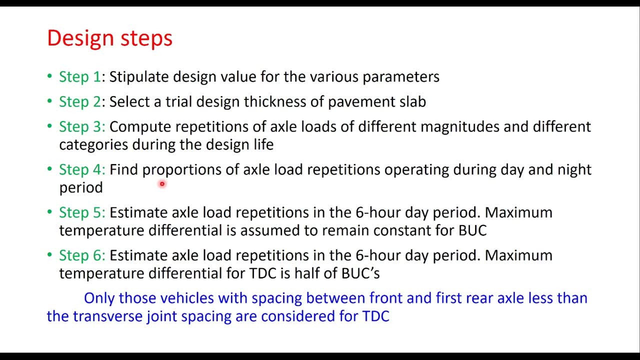 the design is safe. Otherwise we have to change the thickness of the slab. So, in brief, the design steps which are to be considered for design of a concrete pavement are as follows. Step 1 is that you stipulate design values for base parameters. 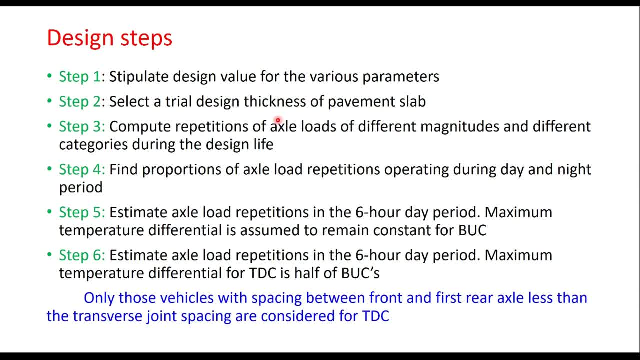 Then select a trial design thickness of pavement slab, Compute repeated number of axle loads of different magnitudes and different categories during the design life And find proportions of axle load repetitions operating during day and night period And from this you estimate axle load repetitions in a 6-hour day period. 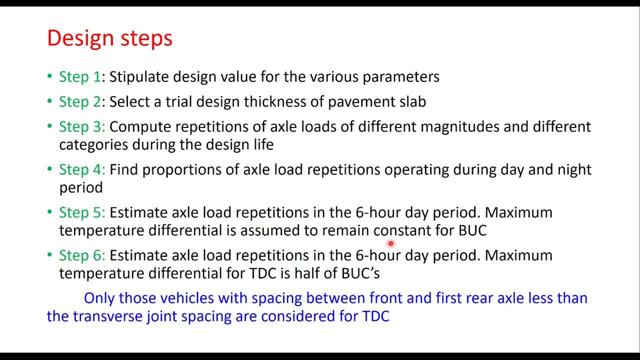 And maximum temperature differential is 0. And maximum temperature differential is assumed to remain constant. for BUC. Estimate axle load repetitions in the 6-hour day period And maximum temperature differential for TDC is half of BUC. You should remember that only those vehicles with spacing between front and first rear axle 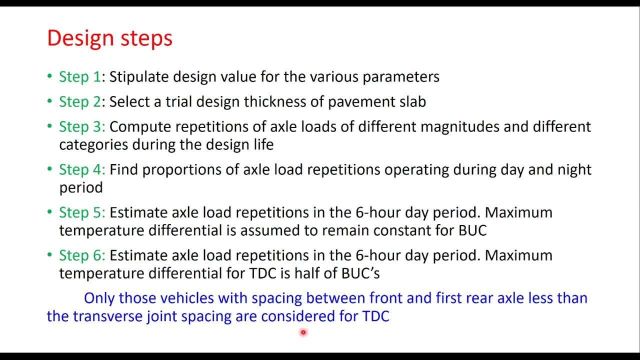 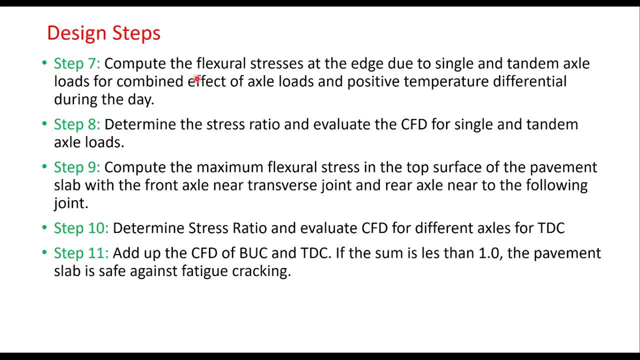 less than the transverse joint spacing are considered for top-down cracking, And this I have explained earlier. also. Step 7 is that compute the flagell stresses at the edge due to single and tandem axle load for combined effect of axle load and positive temperature gradient. 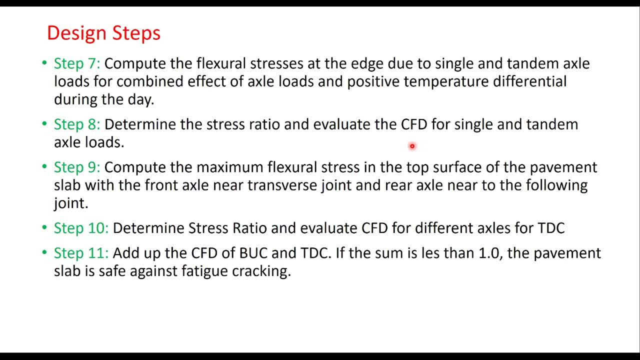 Determine the stress ratio and evaluate the CFD for single and tandem axle loads. Compute the maximum flagell stress in the top surface of the pavement with front axle near transverse joint and rear axle near the following joint. That means the two axles should be close to the joints. 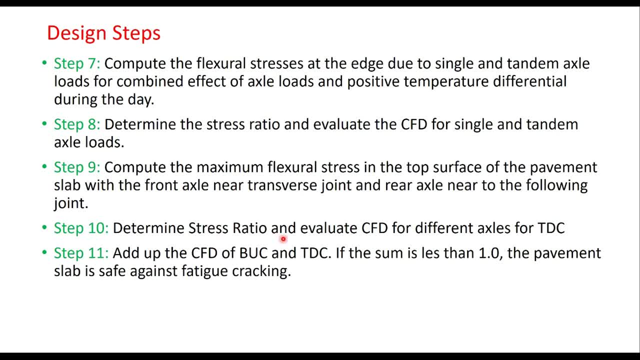 And step 10 is determine the stress ratio and evaluate CFD for different axles for top-down cracking. Add up the CFD of BUC and TDC And if the sum is less than 1, the pavement is safe against fatigue cracking. 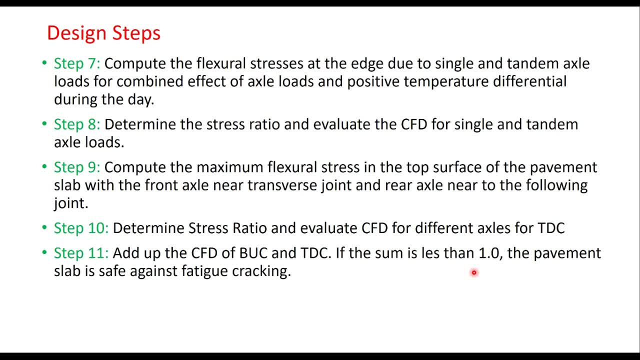 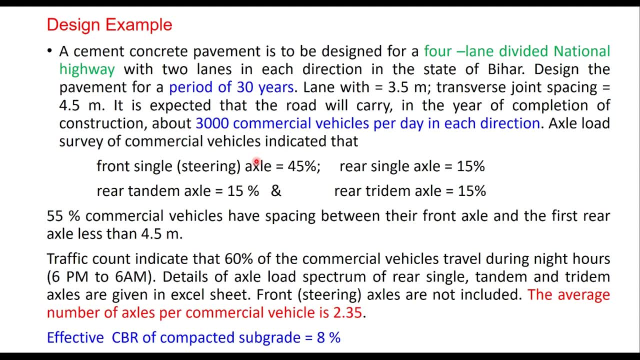 If it is more than 1, then increase the pavement thickness. Now let me explain this procedure, complete procedure- with one example. Then the example is like this: A cement concrete pavement is to be designed for a four-lane divided national highway with two lanes in each direction in the state of Bihar. 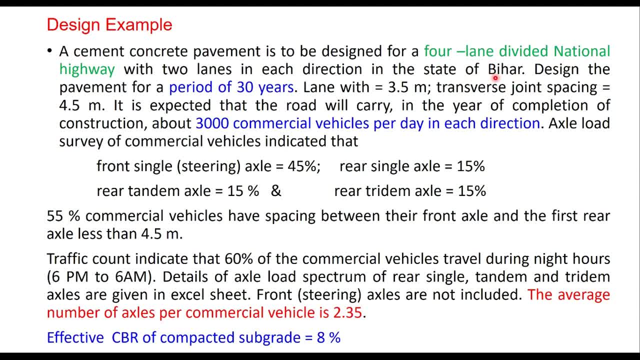 Now. this is required for finding the temperature gradient. Design the pavement for a period of 30 years. Lane width: 3.5 m. transverse joint spacing: 4.5 m. It is expected that the road will carry in the year of completion of construction. 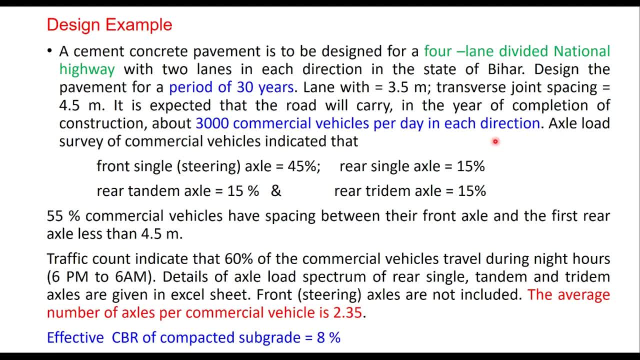 about 3,000 commercial vehicles per day in each direction. Accel load survey of commercial vehicles indicated that front single axle is 45%, rear single axle 15%, rear tandem axle 25% and rear tri-dump axle 15% And 55% commercial vehicles have spacing between their front axle and the first rear axle less than 4.5 m. 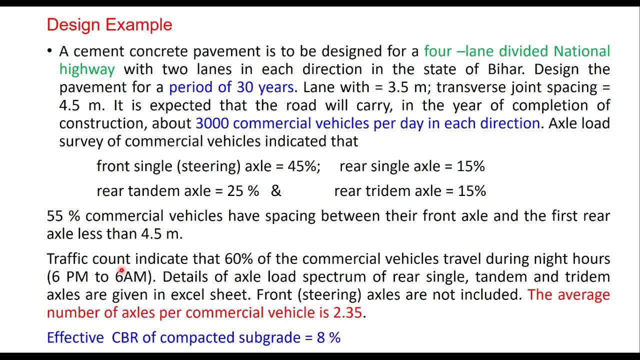 This is the transverse joint spacing. Traffic count indicate that 60% of commercial vehicles travel during night hours, That is, from 6 pm to 6 am, And details of axle load spectrum of rear single tandem and tri-dump axles are given in the axle sheet. 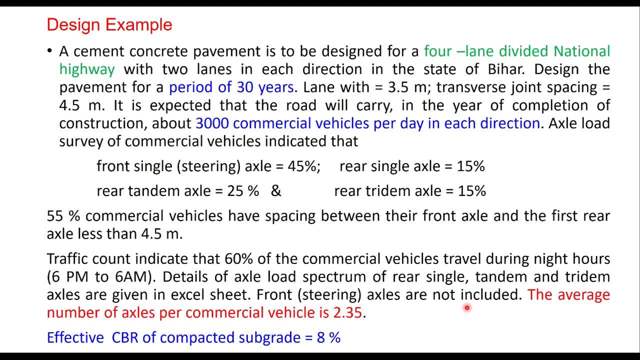 The front axles are not included here. The average number of axles per commercial vehicle is 2.35.. It is more than 1 because of tri-dump axles, And effective CBR of compacted subgrade is taken as 8%. 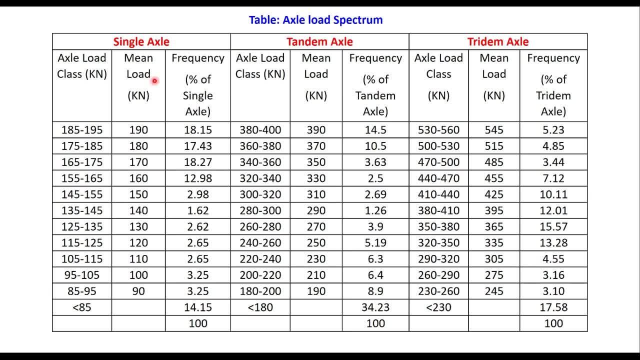 This is the axle load spectrum for single axle, tandem axle and tri-dump axle. The class interval for single axle is generally taken as 10 kN, For tandem axle 20 kN And for tri-dump axle 30 kN. 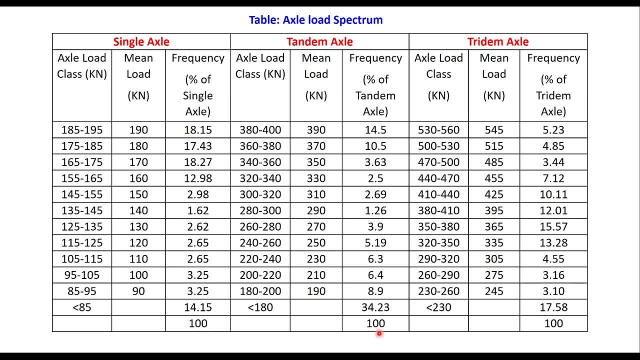 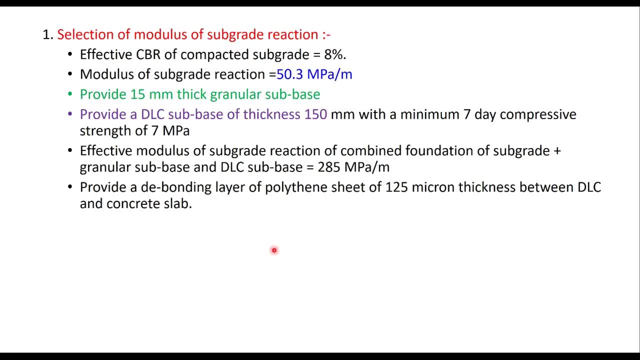 And this is the frequency in percentage, total being 100.. Now this is to be used for cumulative fatigue damage analysis. So the first step in the design is selection of modular subgrade reaction. The effective CBR of compacted subgrade is given 8%. 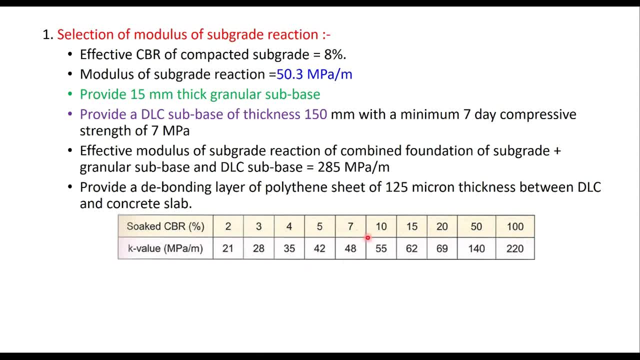 And from this table you can interpolate the value of k between 7 and 10. And you get a value of 50.3 MPa per meter. Let us provide 15 mm thick granular subbase And, above that, a DLC layer of 150 mm thickness with minimum 7-day compressive strength of 7 MPa. 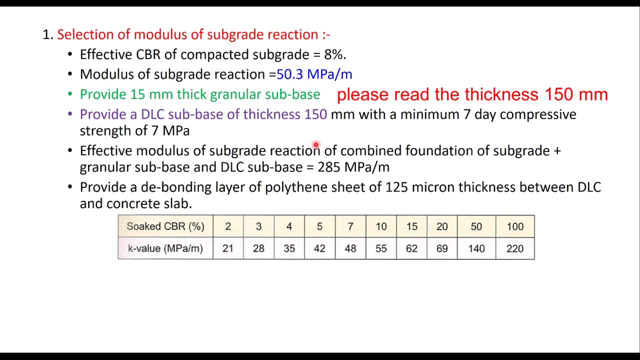 That is the minimum strength required for DLC And therefore effective models of subgrade reaction, of combined foundation, of subgrade plus granular base, and DLC subbase is from this table For a 50.3 MPa per minute and a layer thickness of 150 mm of DLC. 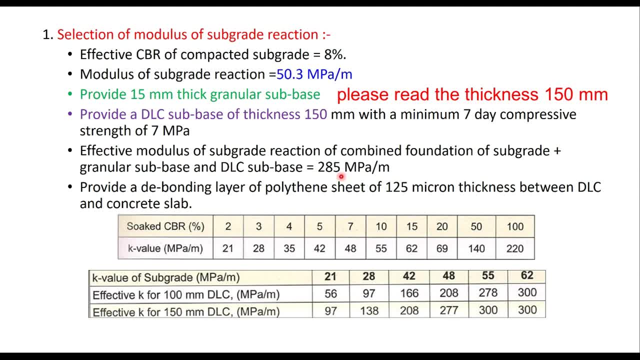 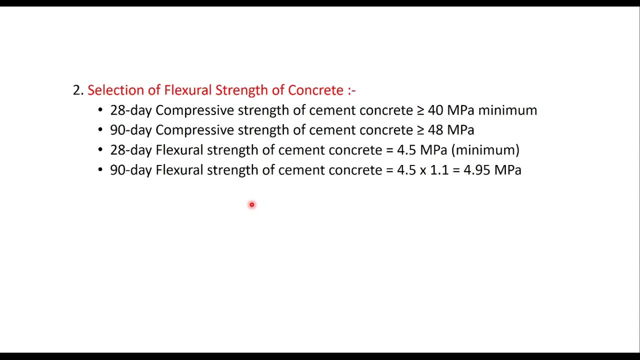 you can interpolate between these- and it will be 285 MPa per meter. Provide a debonding layer of polythene sheet of 125-micron thickness between DLC and concrete slab for smooth surfacing, And the concrete to be used is of M40 grade. 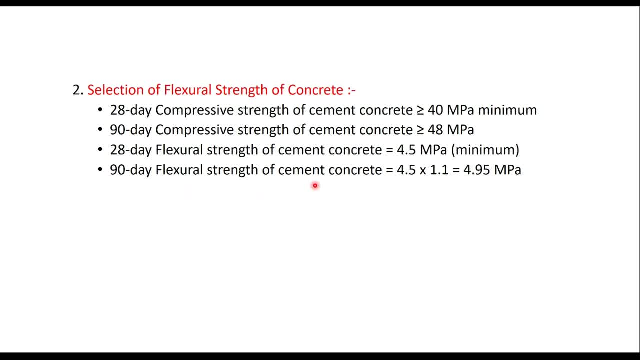 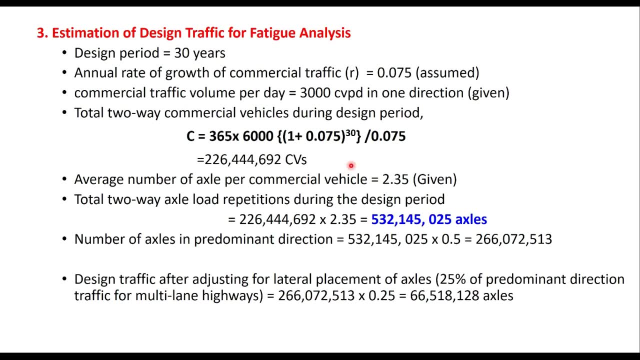 with 90 days of flexible strength of cement concrete: 4.95 MPa. Now we estimate the design traffic for fatigue analysis. Design period given in the question is 30 years. Annual rate of growth: let us assume 0.075 or 7.5%. 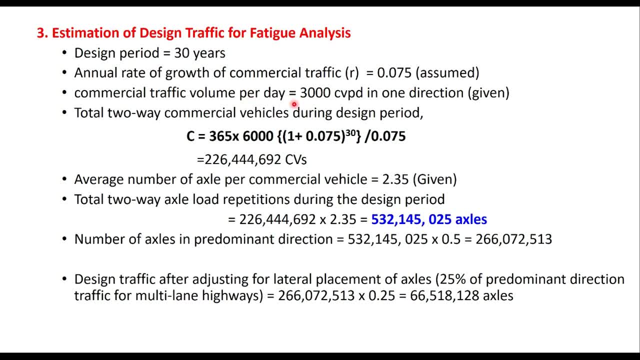 The commercial vehicle per day in each direction is given 3000 commercial vehicles per day And therefore total two-way commercial vehicles during design period will be 365 into A1 plus R power N divided by R, So it is 226,444,692 commercial vehicles. 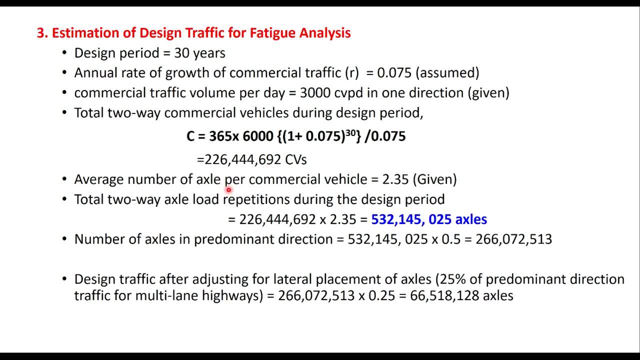 Now, average number of axle per commercial vehicle given is 2.35.. Total two-way axle load repetitions during the design period will be this value multiplied by 2.35,, that is, 532 million axles And the number of axles in predominant direction. 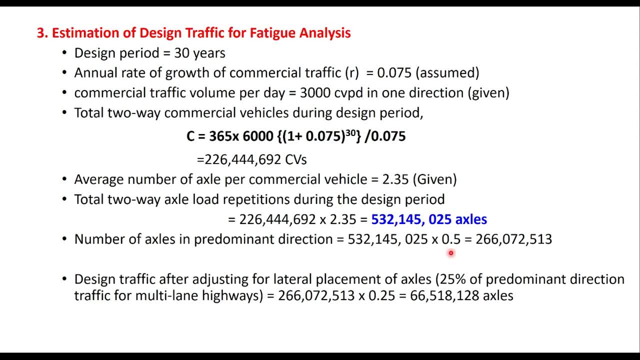 here we assume it is equal in both directions and therefore half of this will be the number of axles in one direction: 266 million Design traffic after adjusting for later placement of axles which is taken as 25% of predominant direction traffic. 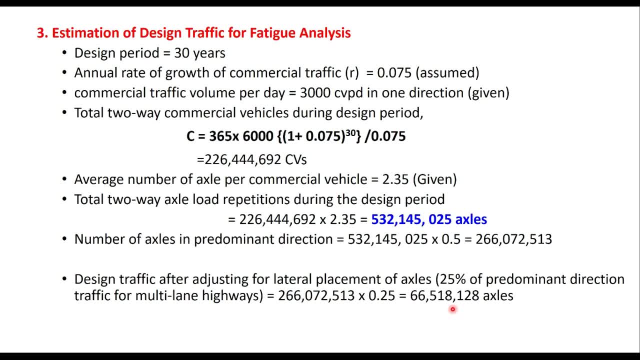 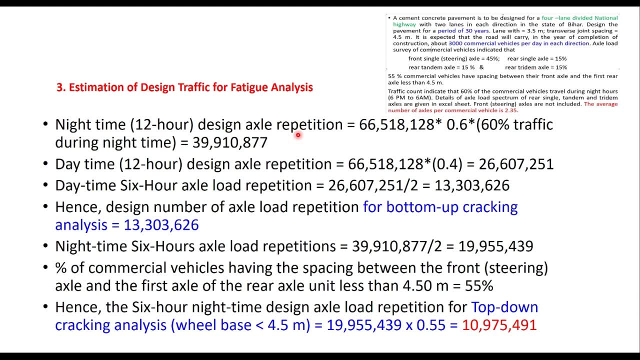 that is 66,518,128 axles. The night time, that is 12 hour, design axle repetition is given as 60% in the question. Total traffic count indicates that 60% of commercial vehicles travel to the night hours. this is the question. 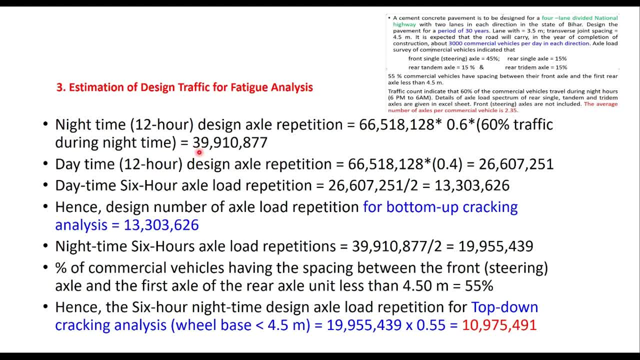 So 60% of this design traffic will be 39,910,877.. Day time: 12 hour will be remaining 40% of this value, that is, 26 million. Now, day time 6 hour: axle load repetition will be half of this: 12 hour repetition. 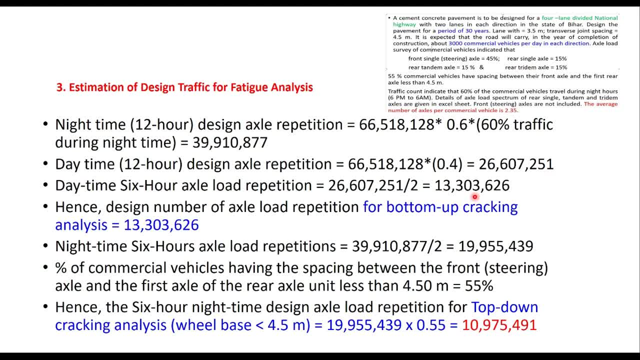 that is half of 26 million 13,303,626.. That is the design traffic for bottom-up cracking. Similarly, night time, 12 hour axle repetitions are 39 million and half of that will be 6 hour load repetitions. 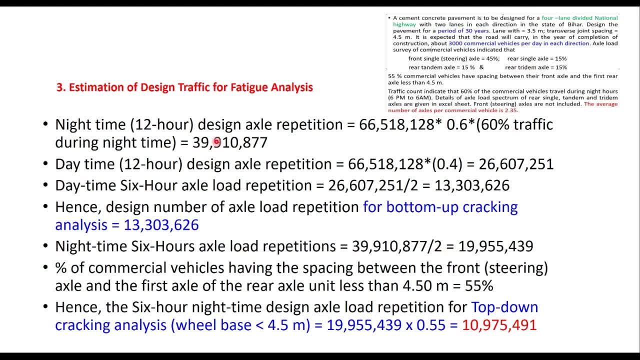 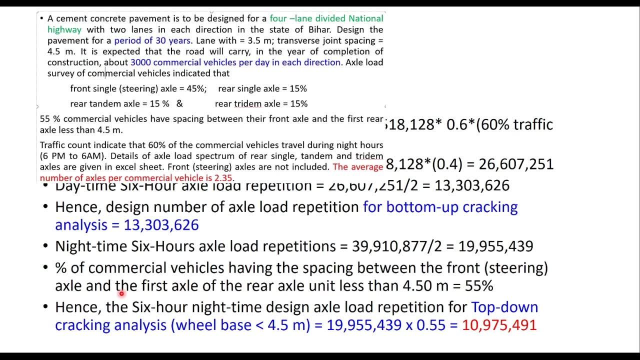 that is 39 million. multiplied by 0.5, that is 19,955,439.. And the percent of commercial vehicles having the spacing between the front axle and the first axle of the rear axle unit less than 4.5 m is 55%. 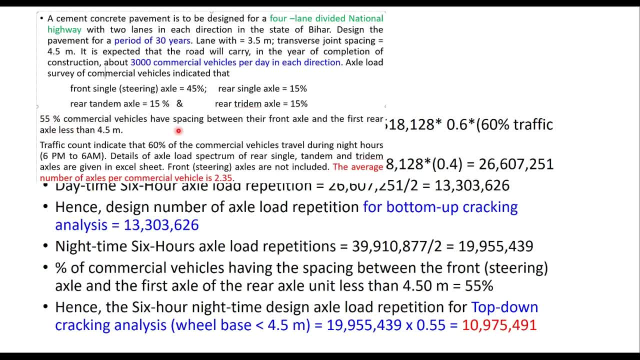 It is given in the question, 55% of commercial vehicles have spacing between their front axle and the first rear axle less than 4.5 m. That is the spacing between the transfer joints. Therefore, the 6 hour night time design axle load repetitions. 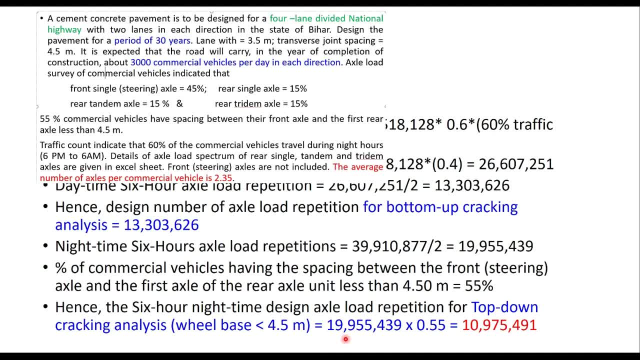 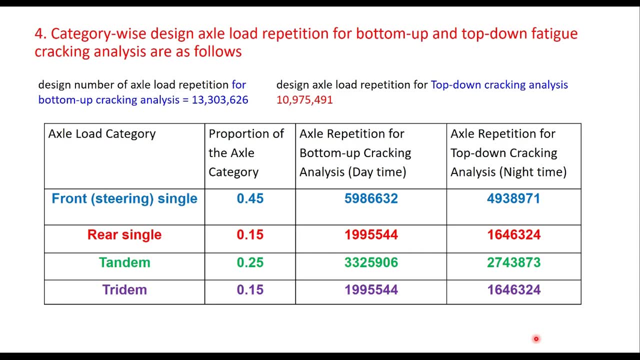 for top-down cracking will be 19,955,439, multiplied by 0.55, that is this value 10,975,491.. So we have the design traffic for bottom-up cracking analysis: 13 million, and for top-down cracking. 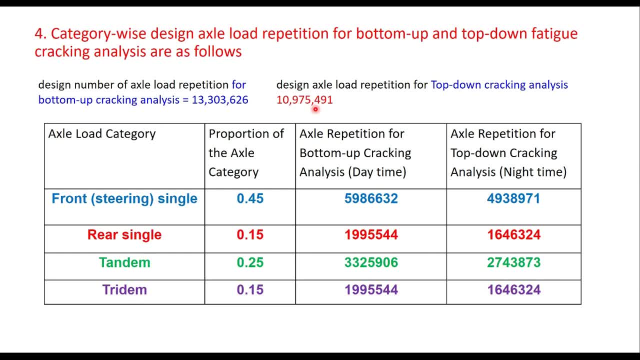 10,975,491.. Now this can be distributed according to axle load category. The front single axle load is 45%, rear single 15%, tandem 25% and tri-dump 15%, given the question, And therefore you can distribute this total traffic. 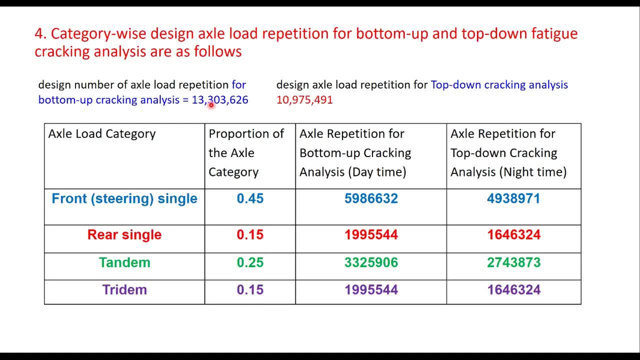 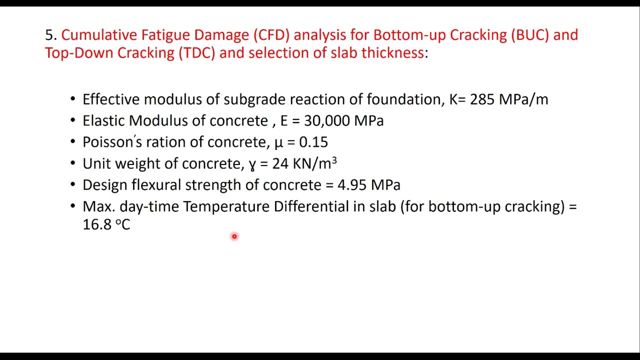 for bottom-up cracking, 13 million to different categories, And similarly for top-down cracking. So this is the design traffic for cumulative fatigue damage analysis. Now we assume some parameters for cumulative fatigue damage analysis: Effective modulus of subgrade reaction. 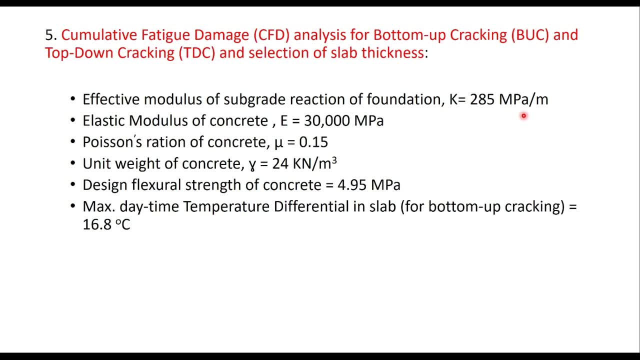 of foundation we have estimated for 285 MPa per meter. Elastic modulus of concrete: for M40 concrete it is 30,000 MPa. Poisson ratio of concrete is taken 0.15.. Unit weight: 24 kiloton per meter cube. 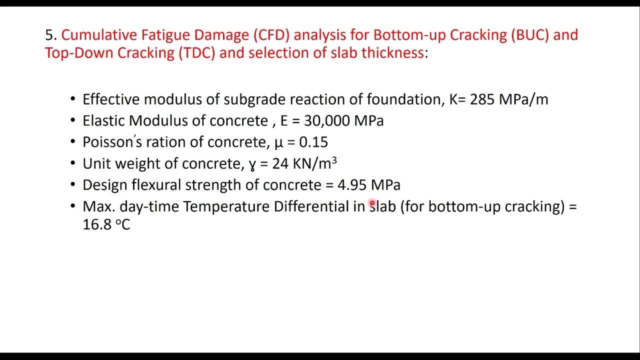 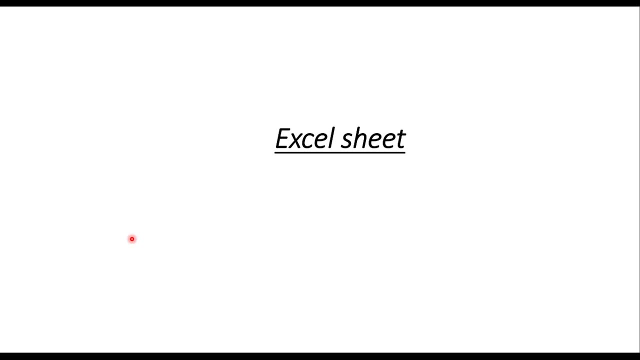 And design strength 4.95 MPa, And for the state of Bihar maximum daytime temperature differential in slab is assumed to be 16.8 degree centigrade. Now, with these parameters, the cumulative fatigue damage analysis is better done in Excel sheet. 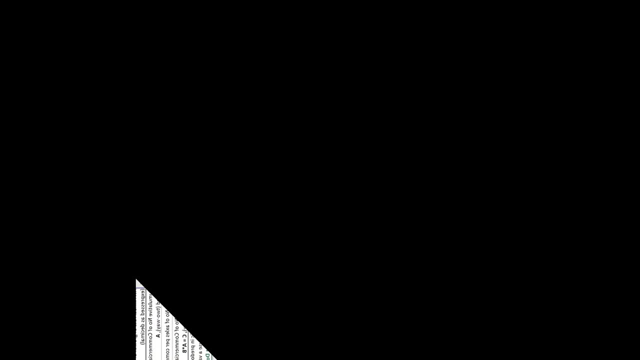 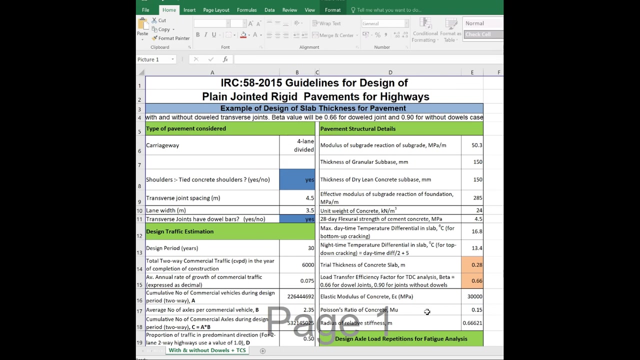 And therefore we now move to Excel sheet. This is the Excel sheet which is used to analyze the pavement. Here, in this part of the Excel sheet, you have all input data like the carriageway, forward lane, divided road transfer, joint spacing 4.5 meter. 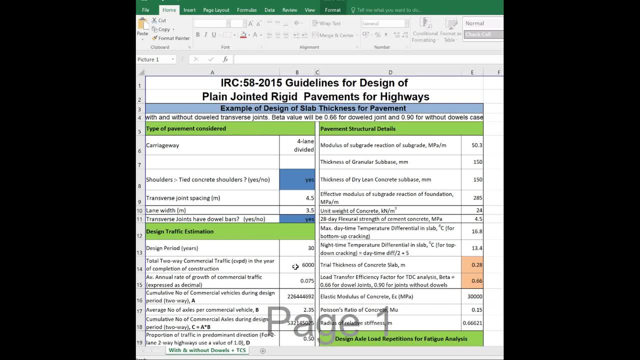 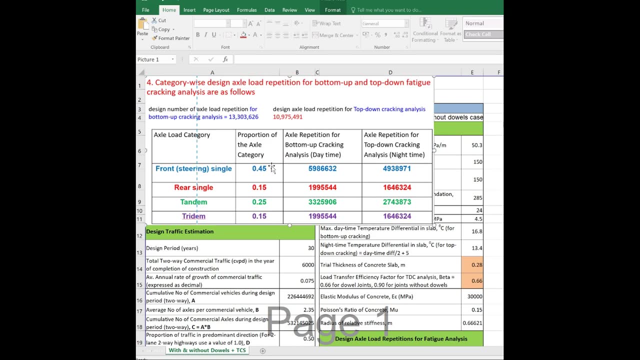 lane width: 3.5 meter. design period: 30 years. number of commercial vehicles: 6,000,. growth rate and so on, And these are the cumulative number of commercial vehicles which we calculated earlier And the information, the figures of interest are these: 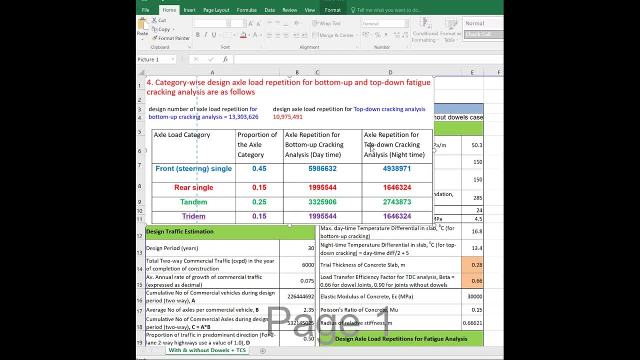 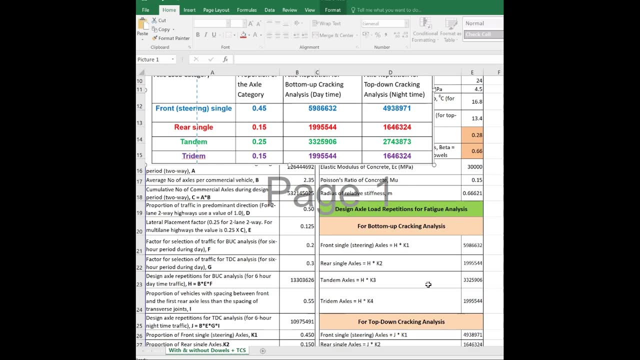 That Excel repetition for bottom-up cracking, Excel repetition for top-down cracking for different types of Excels, And these informations are given here. For bottom-up cracking analysis, you have front single Excel, same value as we calculated here, And for bottom-up cracking analysis, 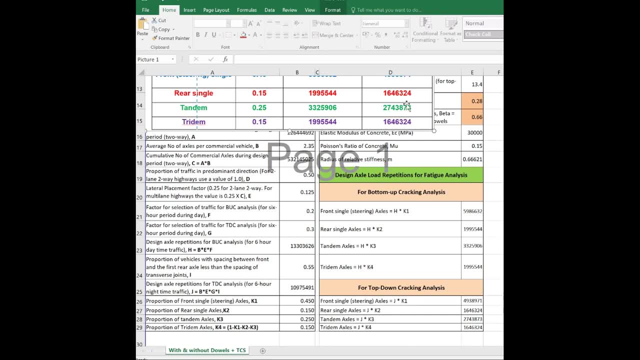 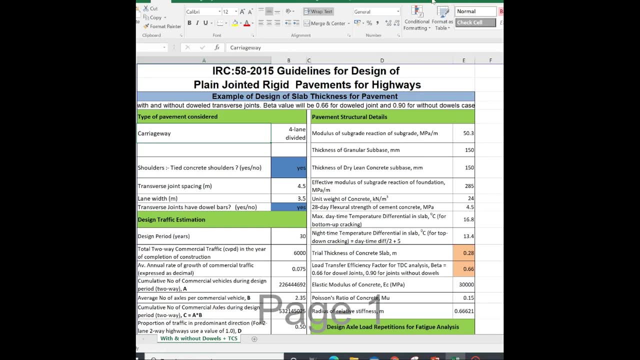 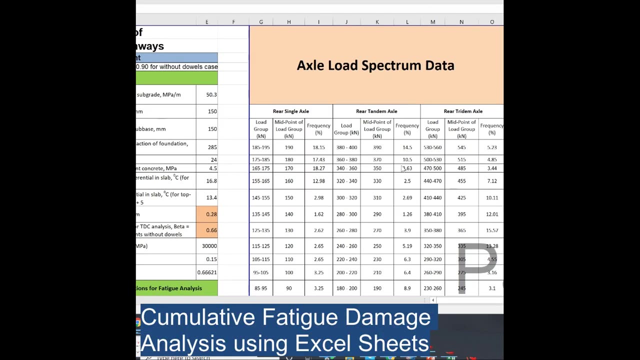 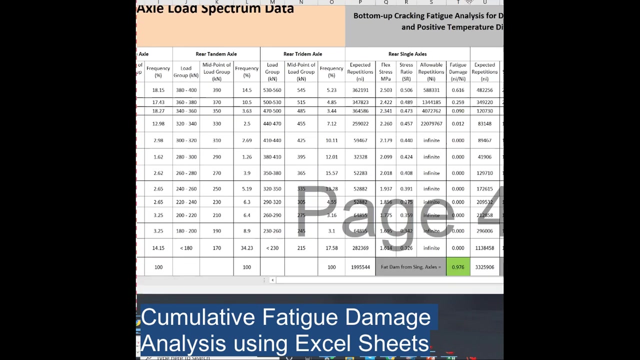 top-down cracking. these values are taken from the list table. Second part of this Excel sheet is Excel load spectrum data, which are also given in the question. These data are used for bottom-up cracking and top-down cracking. For bottom-up cracking: 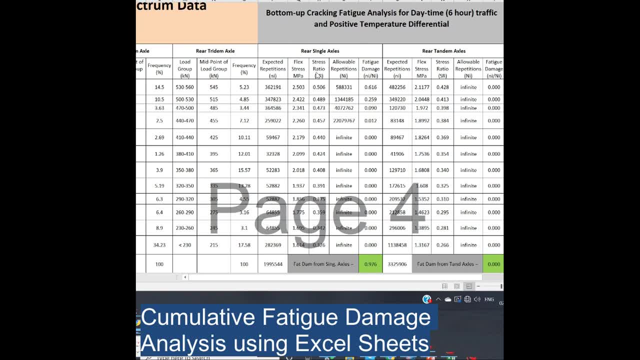 you have rear Excel, rear single Excel. that is expected. number of repetitions: Flexible stress. now this value is calculated using the charts and equations given in the IRC code And this is divided by the flexible stress of the concrete, that is 4.95,. 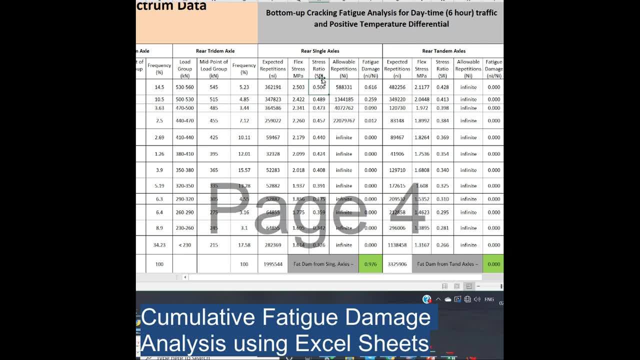 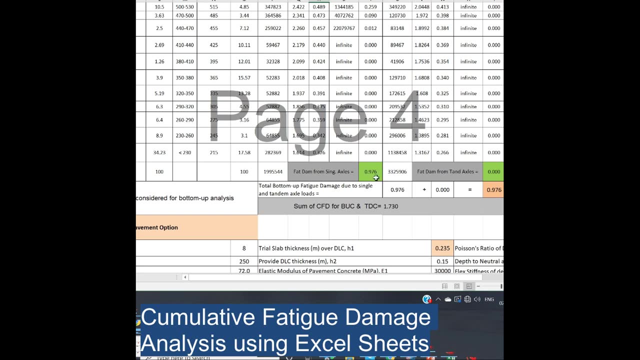 that gives you the stress ratio And, corresponding to this stress ratio, you find out what is the allowable repetitions, And this gives you the fatigue damage. So sum of all these values is 0.976.. Now this is for a assumed thickness of the pavement. 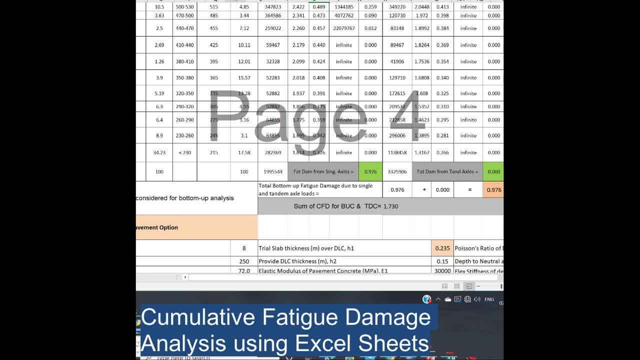 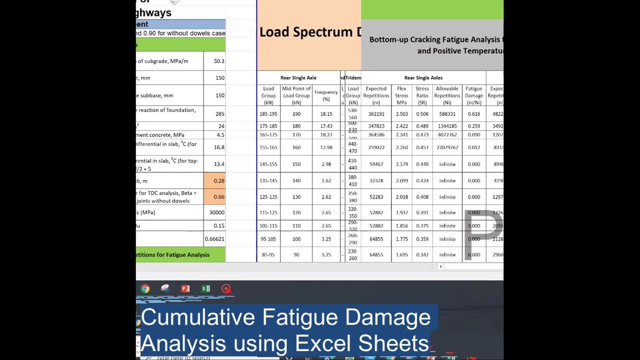 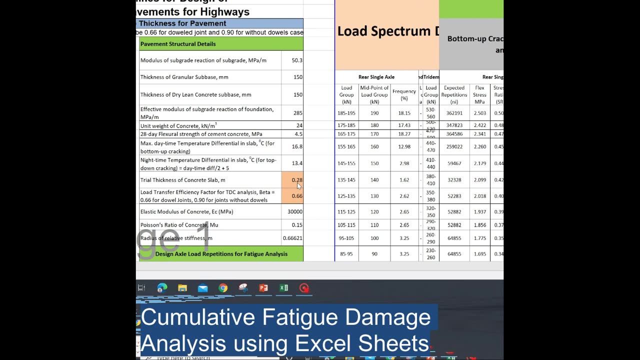 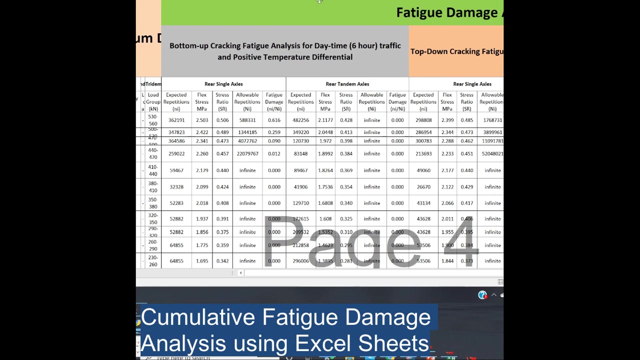 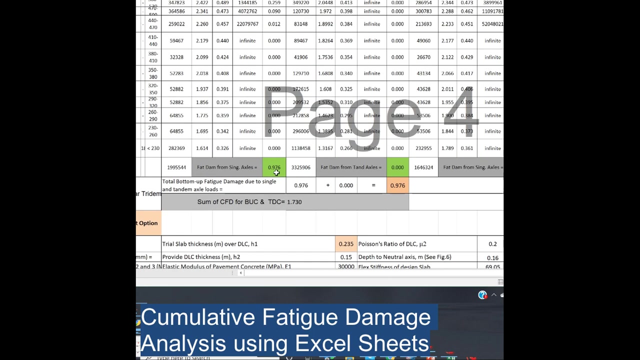 Here I will show you this part that we have assumed initially the pavement thickness to be trial. concrete slab thickness is 28 centimeter. Okay, So for 28 centimeter thickness the fatigue analysis for bottom-up cracking is coming: 0.976 for single Excel. 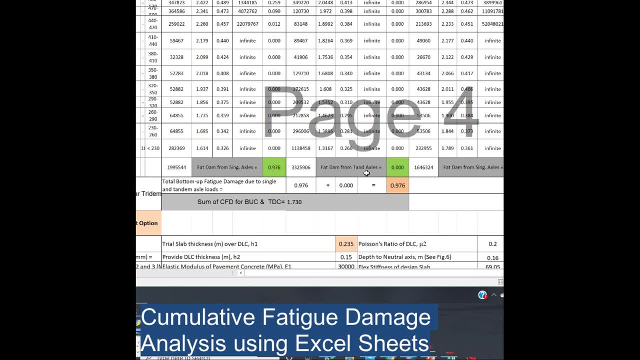 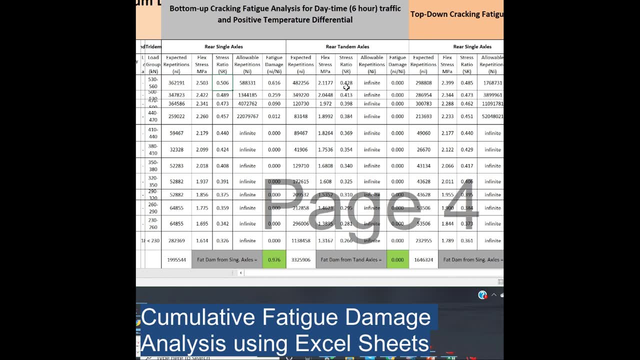 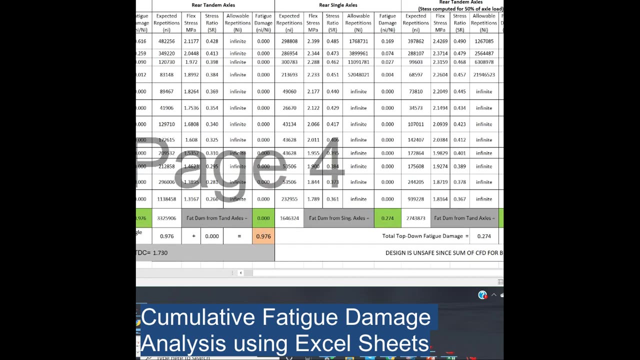 Similarly, for fatigue damage from tandem Excel is 0 because this stress SO is less than 0.45.. And if this value is less than 0.45, the allowable repetitions will be infinite. So there is no fatigue damage For bottom-up fatigue damage. 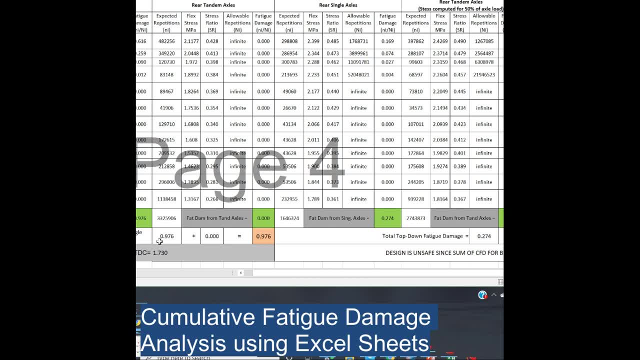 due to single and tandem Excel. load is 0.976 plus 0, that is 0.976.. For bottom-up cracking, I told you we do not consider tri-dome Excels. Similar analysis is done for top-down cracking, But here we consider all three. 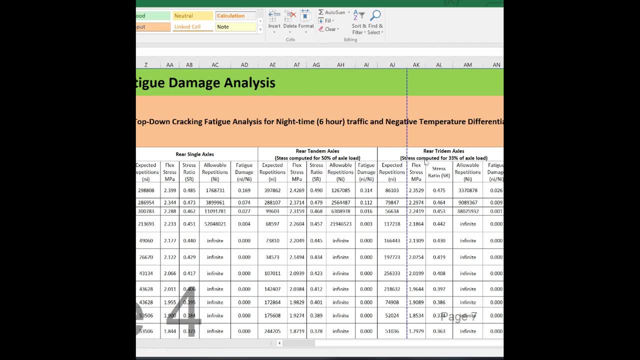 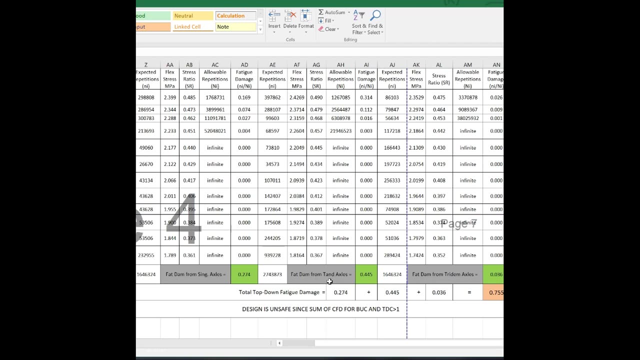 rear single Excels, rear tandem Excels and rear tri-dome Excels. We calculate the fatigue damage and then take sum of all these three. So for single Excel it is 0.274, for tandem Excel 0.445 and for rear tri-dome Excel. 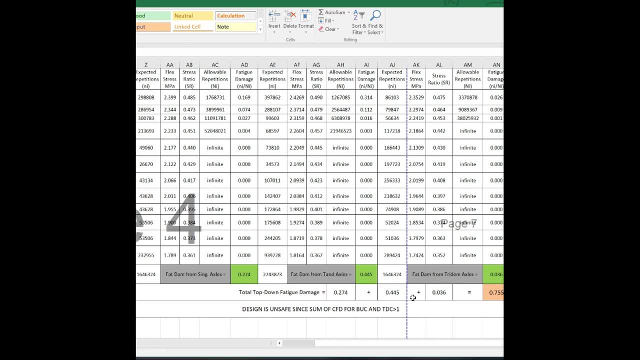 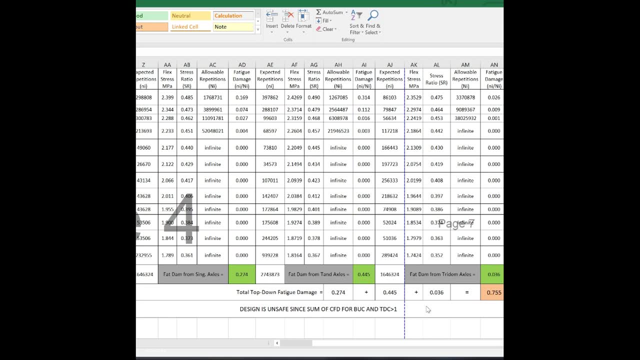 it is 0.036.. So total of these three is 0.755.. Okay Now, since the summation of these two values the total damage because of bottom-up cracking, that was 0.976, and for top-down cracking, 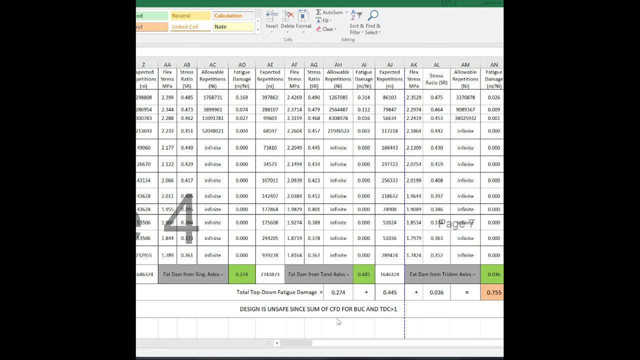 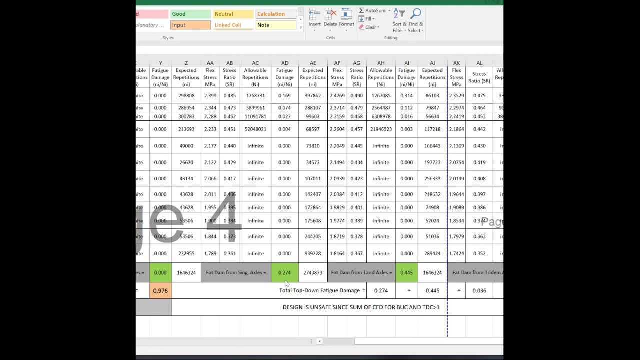 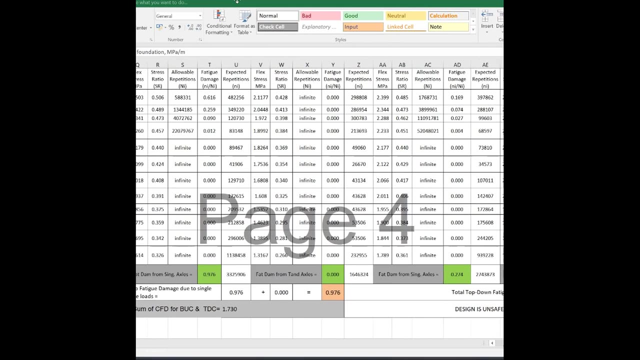 that is, 0.755, is more than 1.. Therefore, this design is not safe. So what we do now? we will change the thickness of the slab. Initially we assumed 28 cm. Let us make it 29 cm. So here in this sheet, 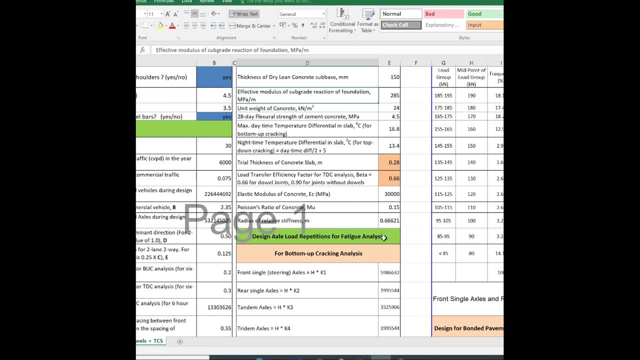 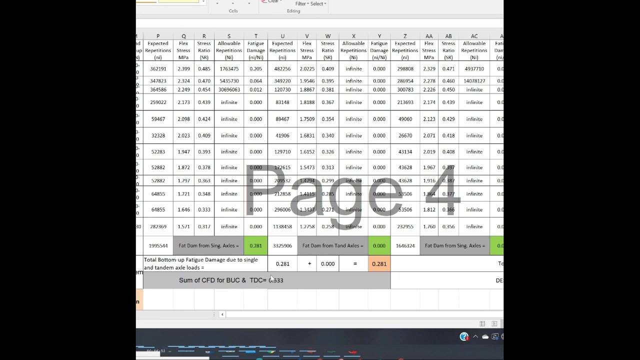 if you assume the thickness to be 20, this thickness, if you change this thickness- trial thickness of concrete slab as 0.29, then all calculations will automatically change and it will give you the sum of CFD for BUC and TDC: 0.533. 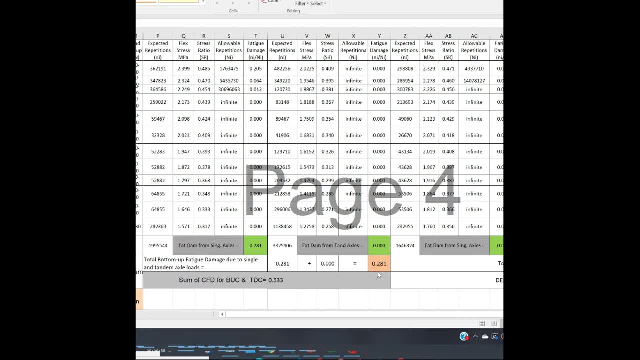 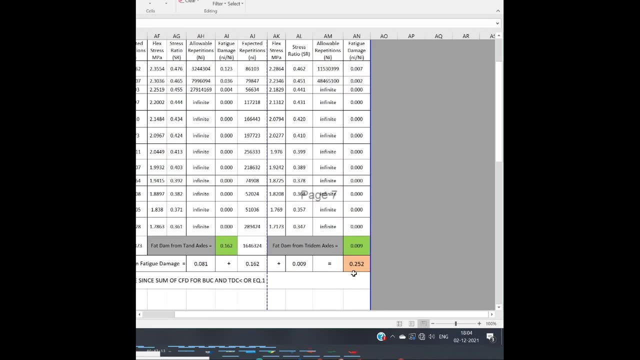 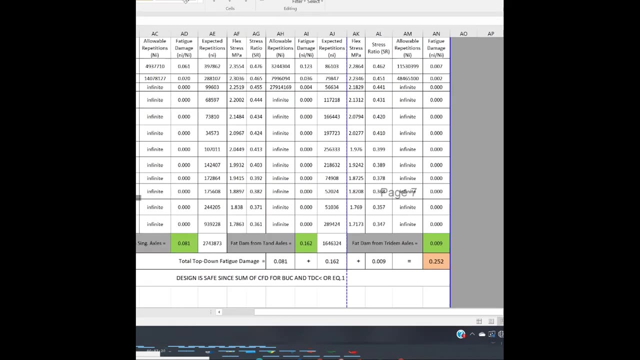 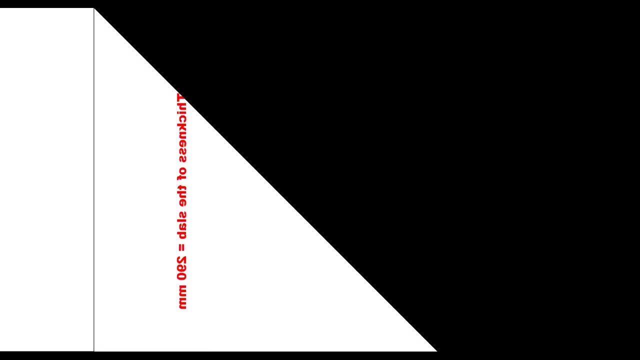 For bottom-up fatigue damage it is now 0.281 and for top-down cracking it is 0.252 and therefore sum is less than 1.. So design is now safe. So it is 0.29 m. So the design thickness of the slab.